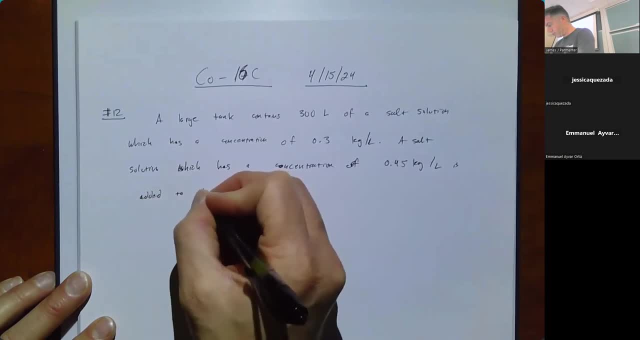 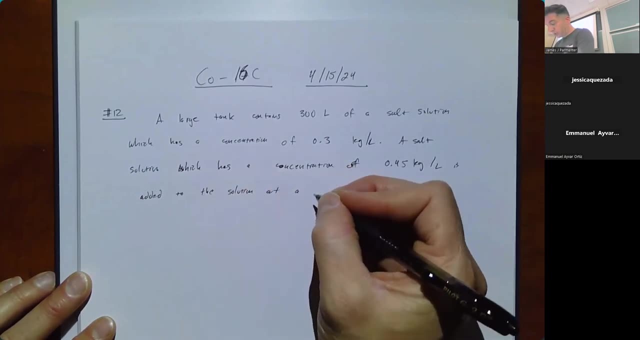 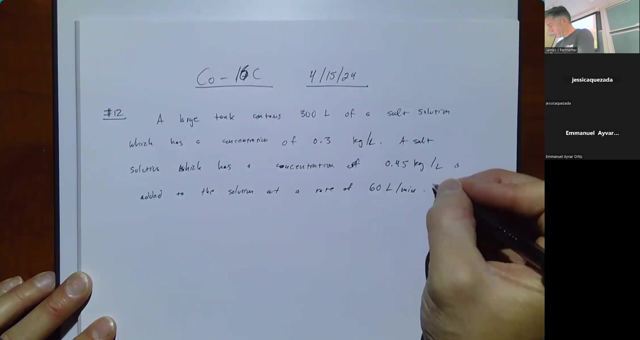 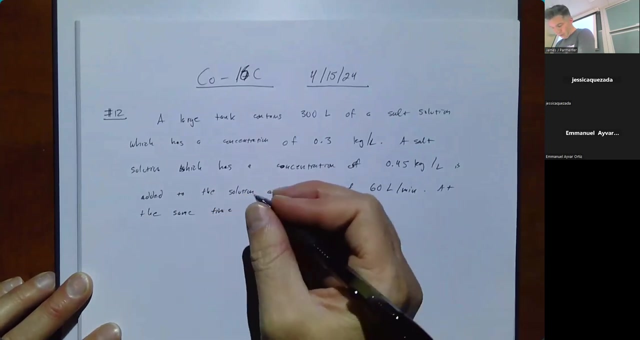 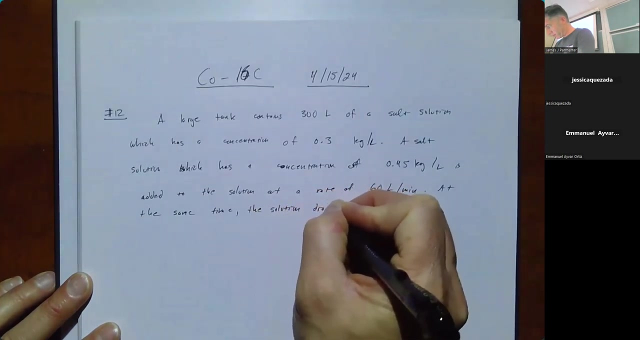 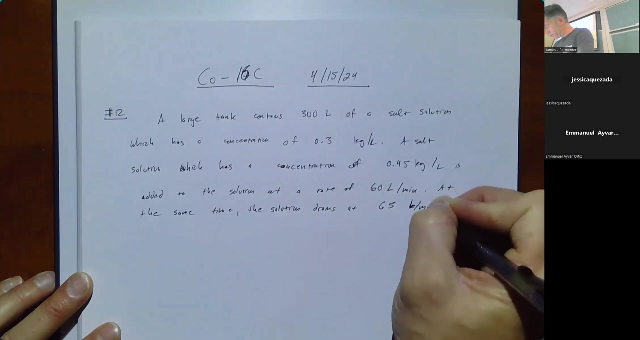 Is added to the solution At a rate of 60 liters per minute. At the same time, It just got darken. At the same time, the solution drains at 65 liters per minute. So we asked you to do two things, but the first part of this is to set up the differential. 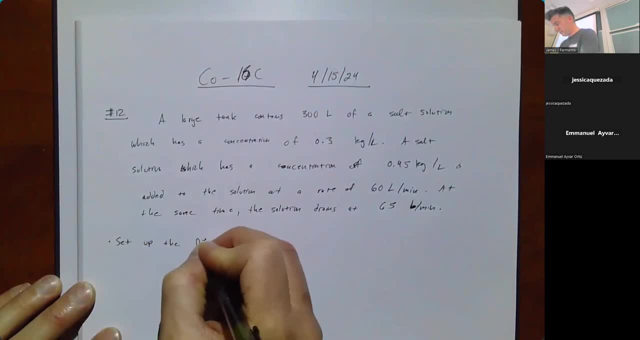 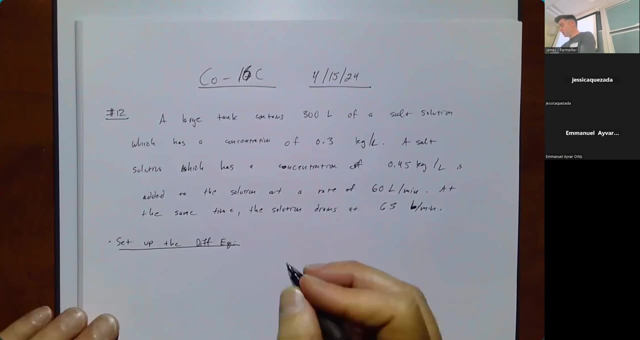 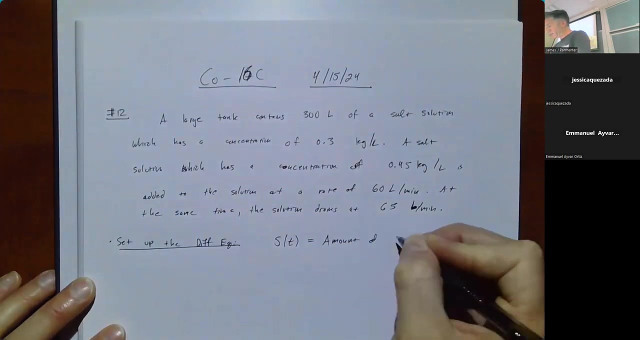 equation. A couple of things here. So we should note that we're going to say that S of T equals- and this is where it's really important to be aware of what we're talking about- not the concentration, but the amount of salt in the tank at time- T. 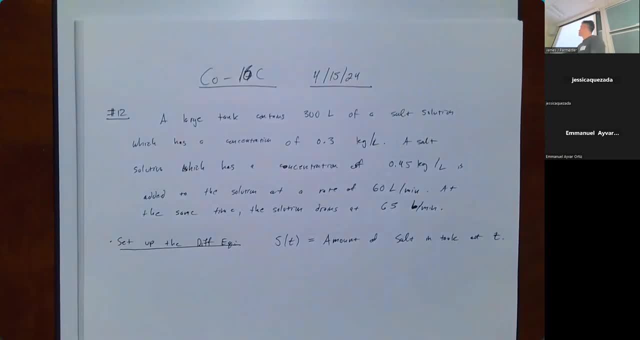 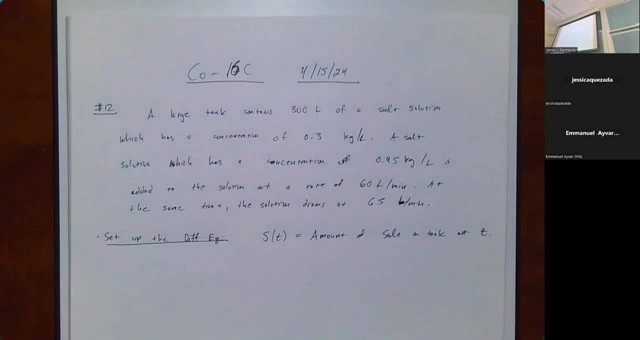 Okay, Yeah, it kind of sorry, just the back. well, it's not going to be too terrible, It's kind of terrible. That is halfway. here's how the front half is even worse. Yeah, halfway is the back, it's the front. it's like two-thirds in the back or one-third. 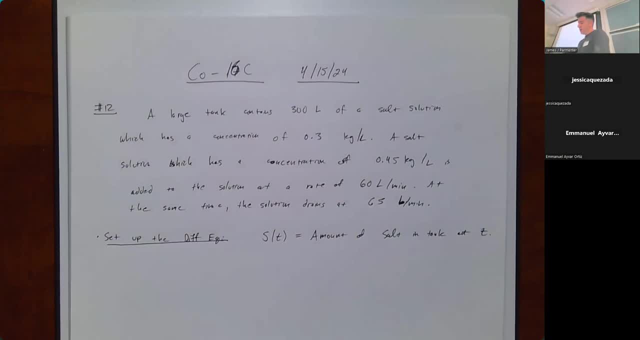 in the front. Yeah, I guess we'll just live with sitting in the dark. So to set up this differential equation, we're going to say that dSdT, that's the rate of change of the amount of S, is equal to. I usually like to write it's the rate in minus. 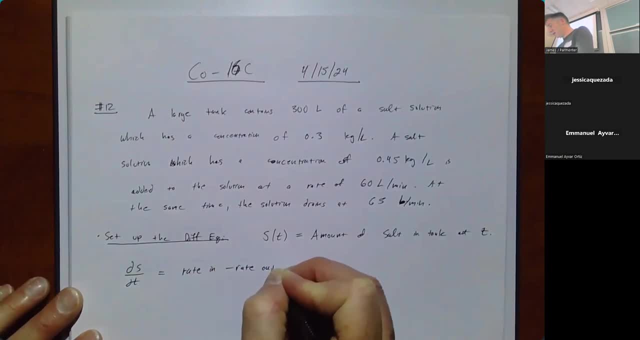 the rate out. I think my teacher's reminding me of the amount in minus the amount out. it's the same idea. It's how much we're putting in minus how much we're taking out. The in part is usually the easier part to deal with, so when I'm thinking about this, 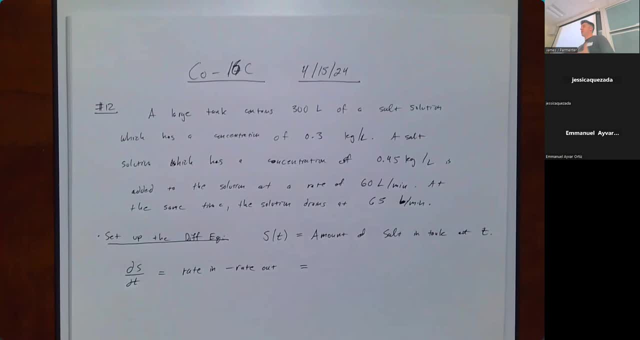 rate in minus rate out. I'm really thinking of it's the concentration of the solution going in times, how fast we're putting that in. So let's see: the concentration that's going in is 0.45 kilograms per liter. 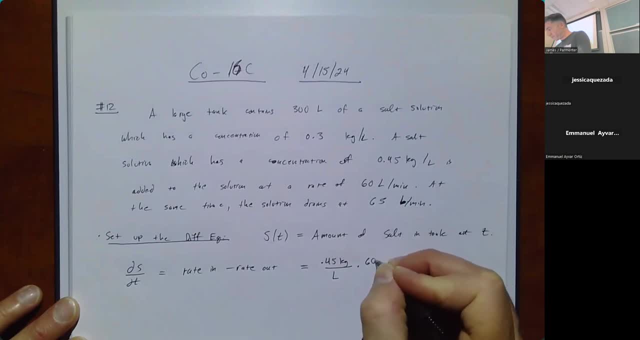 And then we're putting in at a rate of 60 liters per minute. Let me see, there we go. So no, I guess. thank you, So it really doesn't matter. The rate out part here is always the more challenging part. 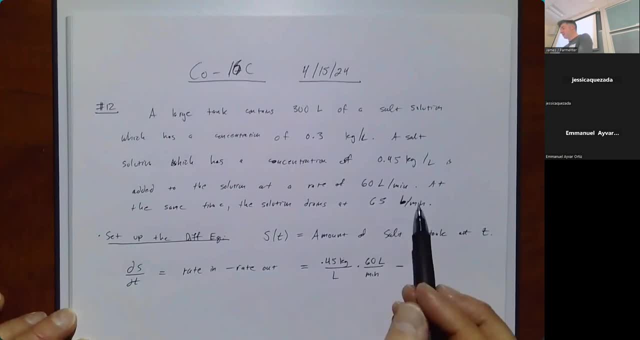 So we know that we're draining this. well, actually, we should talk about the concentration first. So the concentration of the tank is how much salt there is, which is S or S of T, if you prefer, but I'm going to write S. 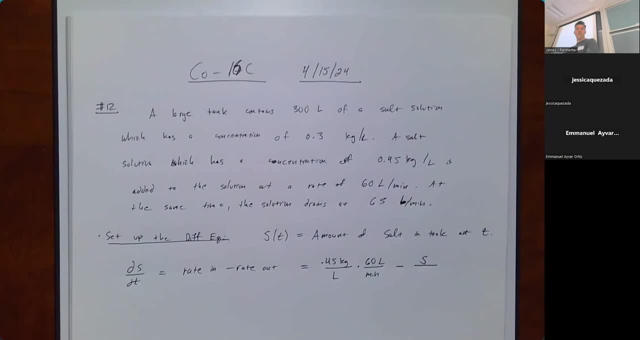 So S kilograms Added by the volume of the tank. and here what makes this different than our previous setups is that the volume of the tank is changing. We're putting solution in at a rate of 60 liters per minute and taking out at 65 liters. 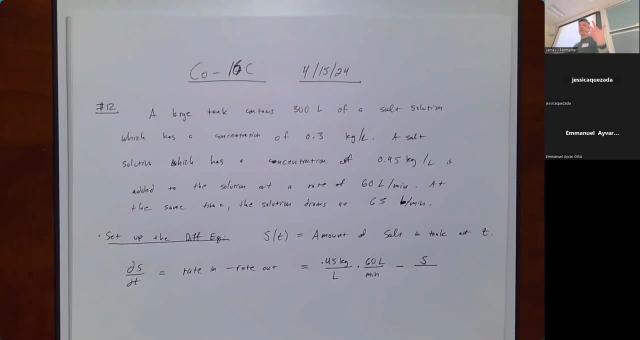 per minute. So every minute we're losing five liters. So we're starting off with an initial volume of 300 liters and then every minute we're going to subtract off five liters. We're going to subtract off five times T, where T is measured in minutes. 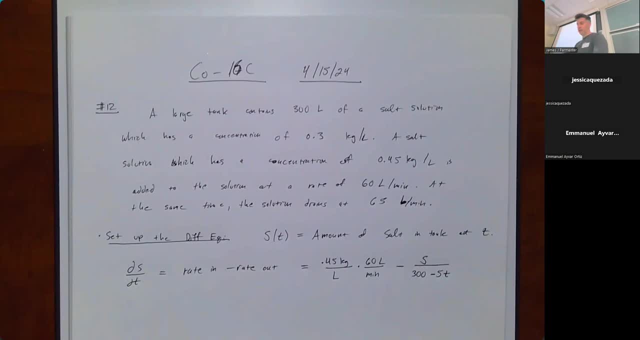 Correct, it's 300 minus five T. And then multiply it by how fast we're taking that solution out, which is 65 liters per minute. Let's do this here, So that's going to end up being the DSDT is equal to T. 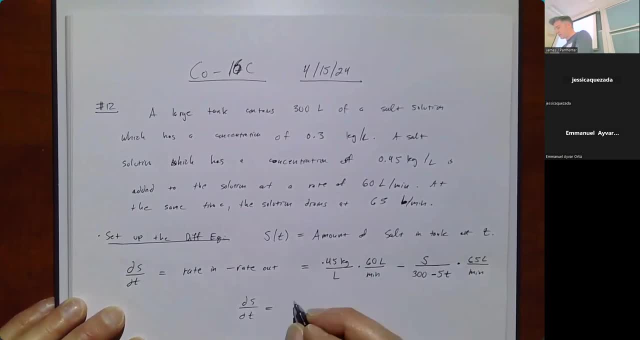 So that's going to end up being the DSDT is equal to T, So that's going to end up being the DSDT is equal to T, So that's going to end up being the DSDT is equal to 0.45 times 60 is 27, minus. I would write this as 65 times S over. 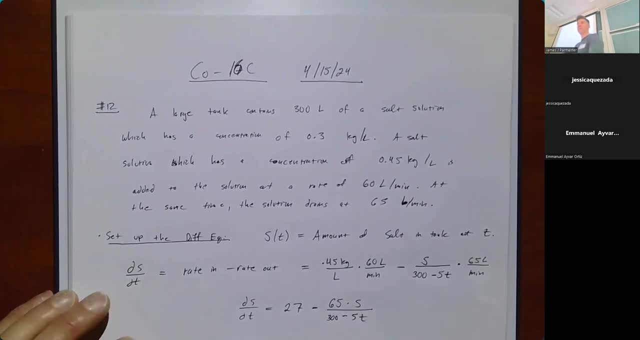 300 minus five T. Yeah, yeah, yeah. So the five is coming from the difference between the 65 liters per minute that's going out and the 60 liters per minute that's going in. So every minute we're going to lose five liters. 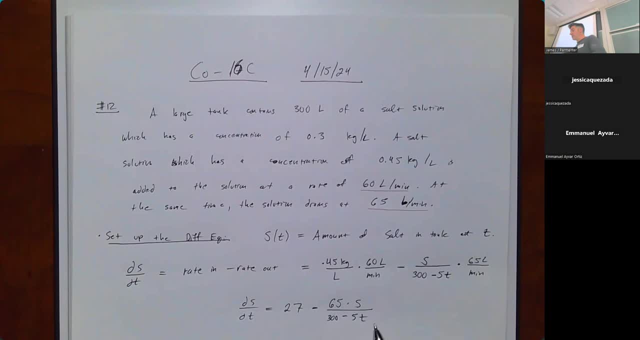 So when t equals 1, we've lost 5 liters, and so the volume is now 295.. When t equals 10, we've lost 50 liters and the volume is 250.. This one, definitely, yeah, definitely. I was about to say definitely, maybe. 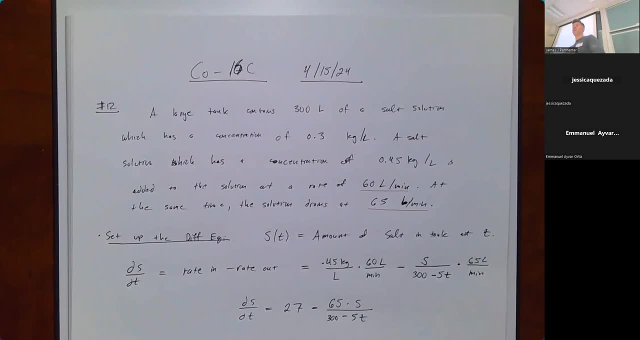 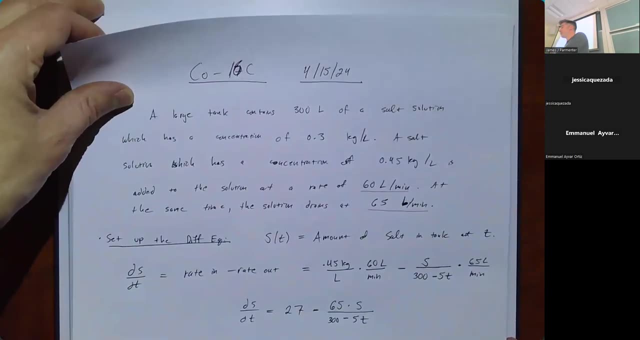 This one probably has to be done with the first-order linear. So we're not going to solve this because it's a little more complicated. But if you were to solve this, let's talk about how you would set up and solve it, although we're not going to finish it probably. 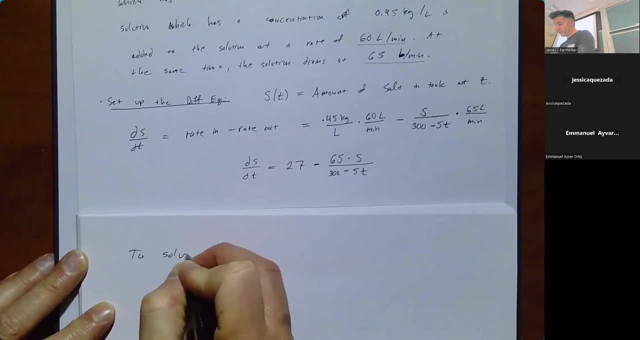 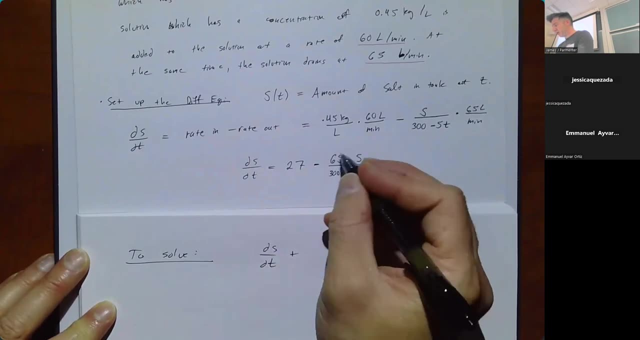 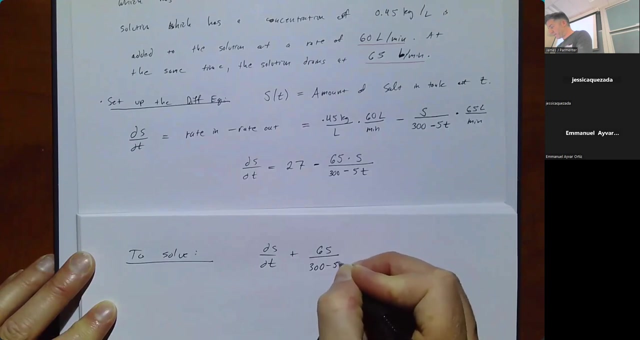 So to solve, we would rewrite this as ds, dt plus this part here, the 65 over. I'm going to write it as 65 over 300 minus 5t, 5t times s, equal to 27.. And so this is the usual kind of setup. 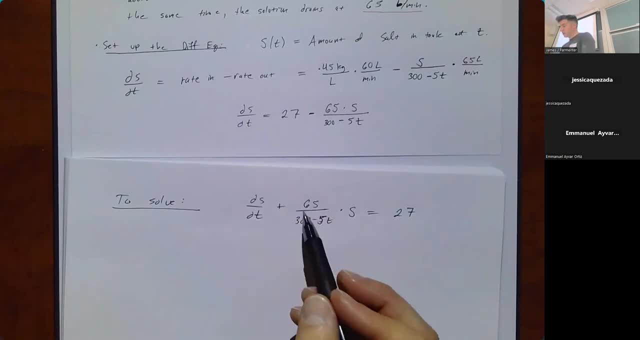 Here's essentially my y prime. Here's my p of t times y, Here's my q of t. So then we would find the integrating factor. Our integrating factor would be e to the integral of that mess there, 65 over 300 minus 5t. 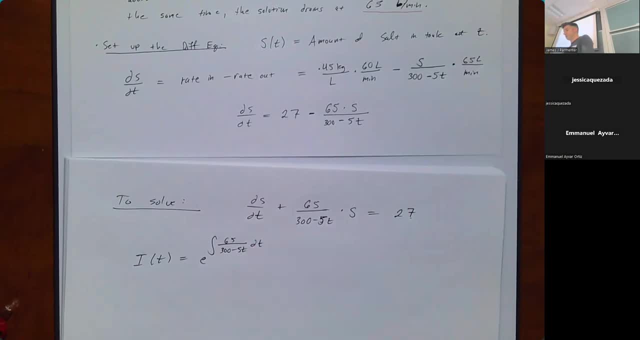 which actually probably isn't too terrible to solve because it ends up being somewhat not too often, But that's not really the point of this question, so I don't think we need to continue with that right now. I will. I want to point out two other things that are asked here. 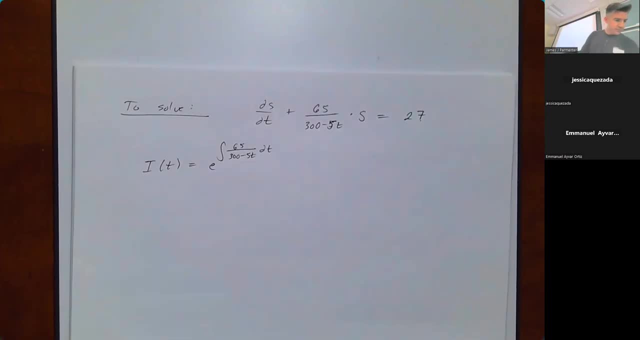 So the first question- So they do ask us at: t equals zero. what is s of zero? And this question is really just getting at making sure that you understand the difference between what s represents and what we're being told. We're being told that the initial concentration of the tank is 0.3 kilograms per liter. 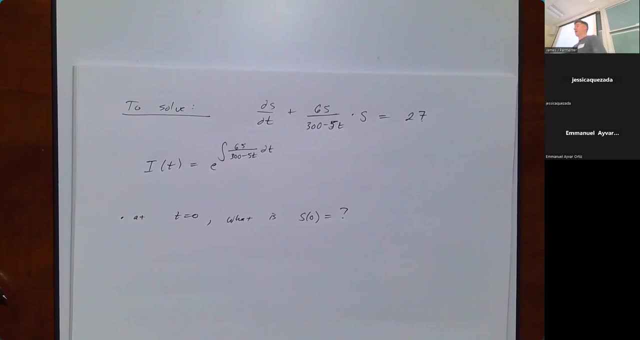 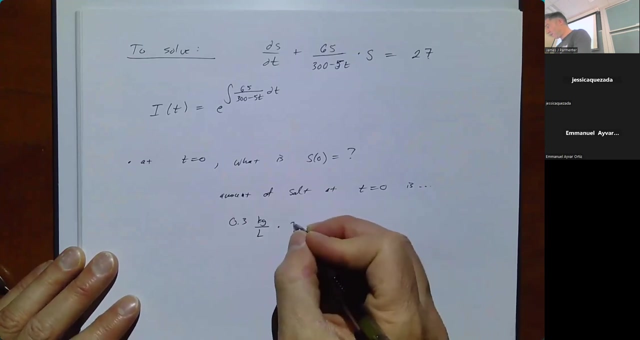 And we're told that the tank initially holds 300 liters of solution. So our s of zero is just going to be the amount of salt at the beginning, which is going to be, well, the concentration of 0.3 kilograms per liter times the total volume. 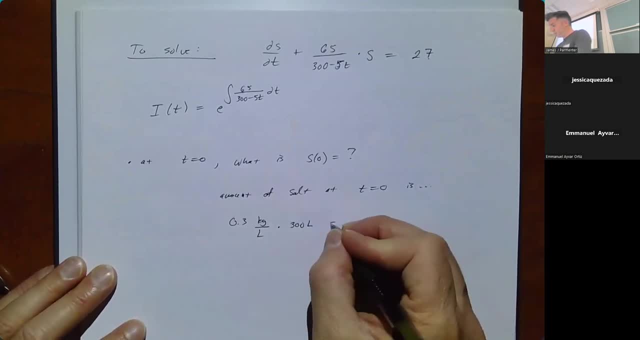 which is 300 liters, which ends up being what? 90? Kilograms of salt. That's what might make that question a little trickier than you might normally think it would be. So again, I'll say this is pretty generally true. 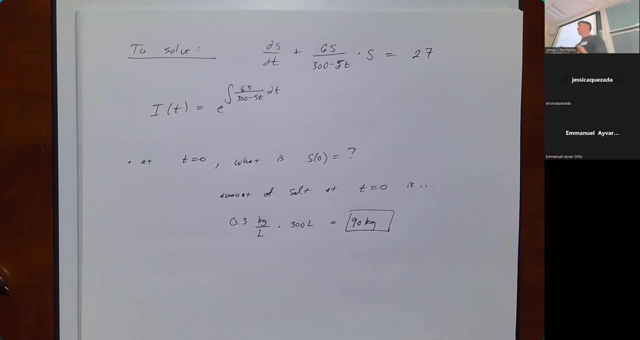 Then when you're talking about these problems, you're always talking about the amount of stuff that you have in the tank or wherever, not the concentration of that stuff. The only other question I could see asking here without actually solving it would be how long. 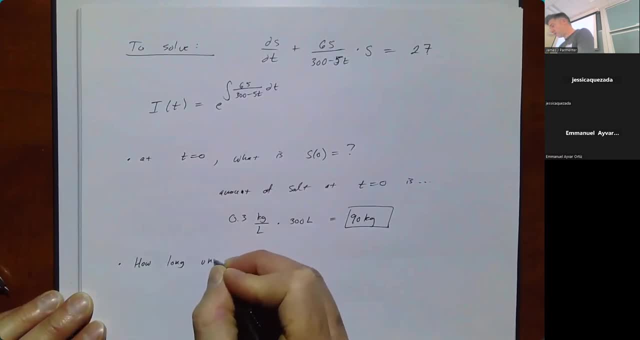 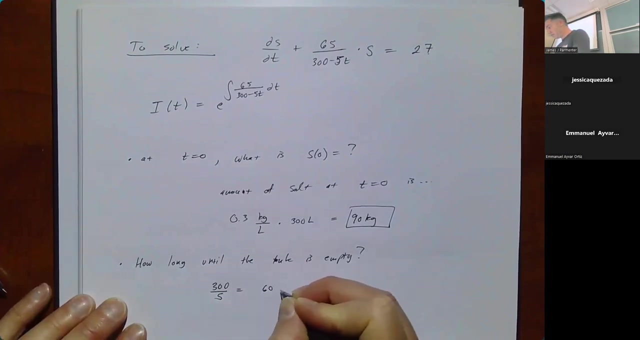 How long does this process continue, or in other words, how long until the tank is empty? Well, we're losing five liters every minute, and the tank started off with 300 liters, So I think we just have to do 300 divided by five, which is going to be 60 minutes. 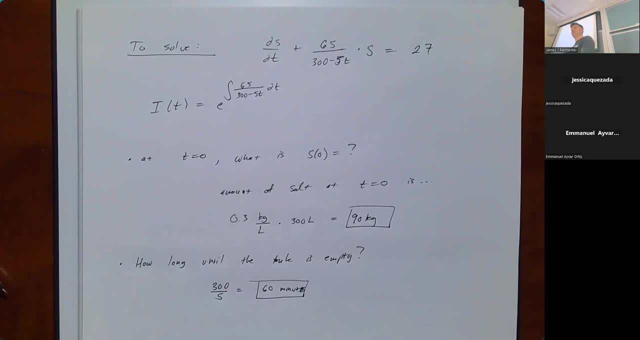 So exactly one hour? Cool Right, because every minute we're losing five liters. All right, Let's look at a couple more word problems, just because people have asked for some more word problems. I really think the hard part about the word problems is the set. 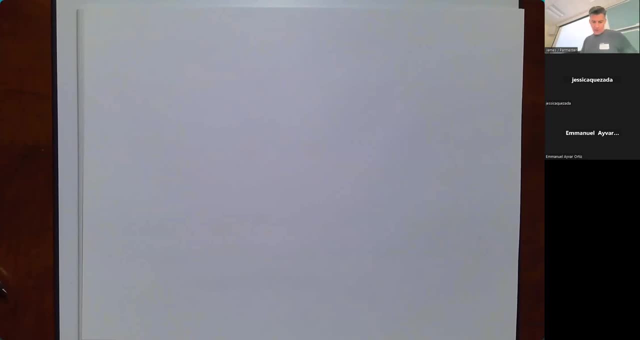 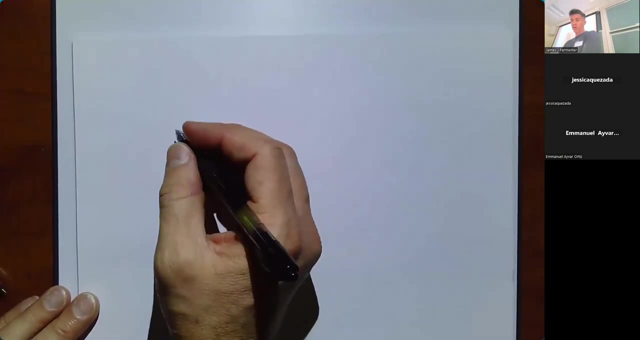 So that's what we're going to focus on right now. So let's look at something like this. So yeah, I am taking problems from the homework just to kind of talk about the setup, not so much the solving. Let's look. 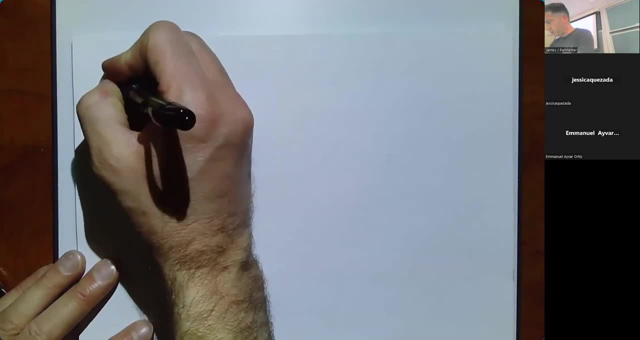 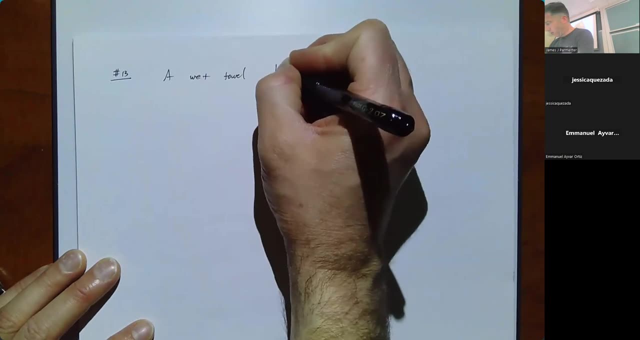 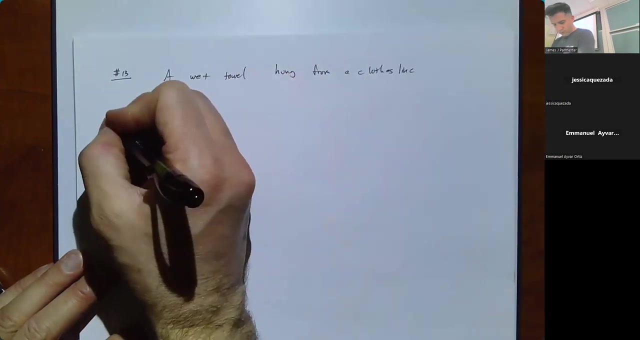 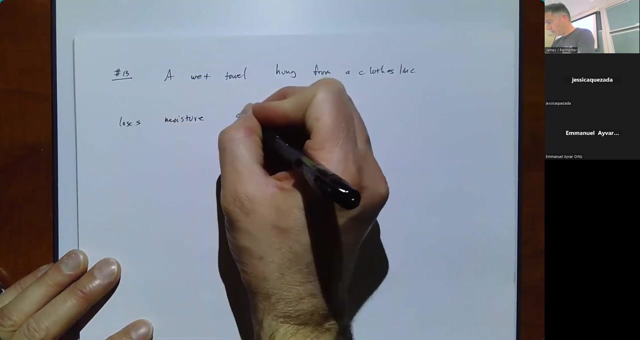 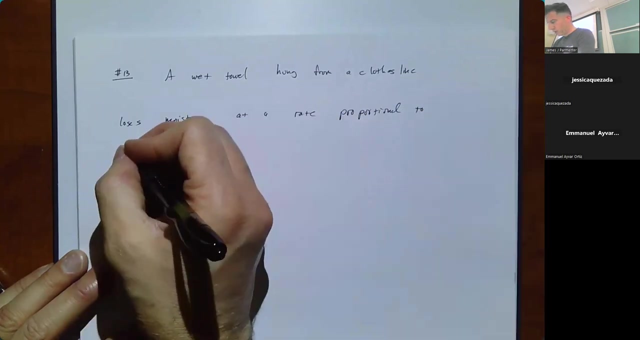 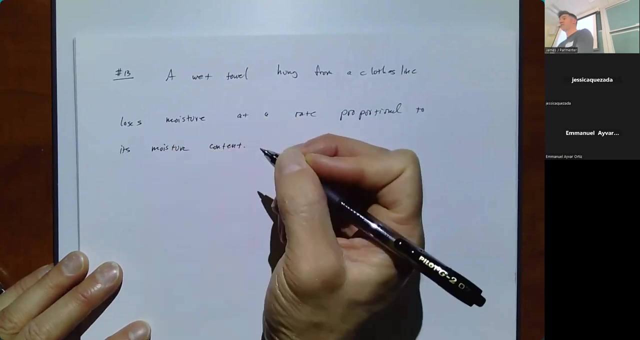 Yeah, Sure, This is number 13.. A wet towel hung from a clothesline loses moisture. That's a real big space there. James Loses moisture at a rate proportional to To its moisture content, Or in other words, the more moist it is, the faster it will lose moisture. The less moist it is, the slower it loses moisture because of proportionality. If, after four hours, The towel has lost 30% of its moisture, How long until it will have lost 50%? I'm going to change that last part. 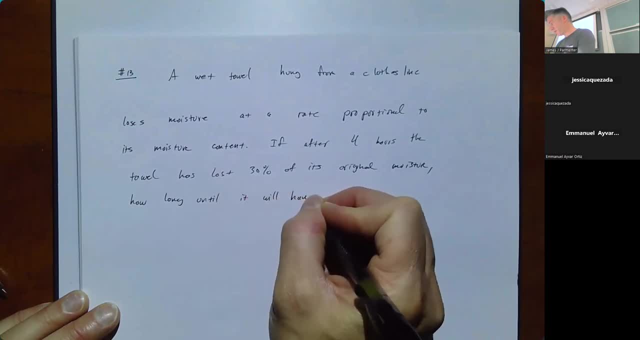 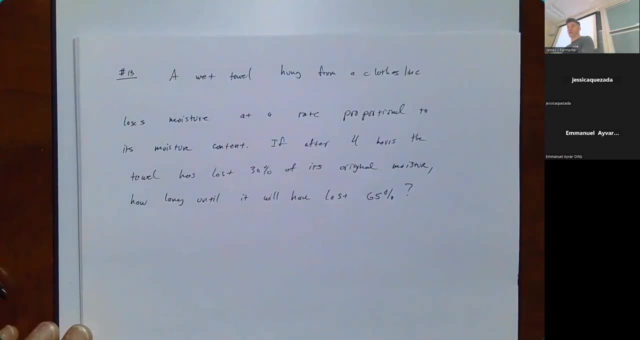 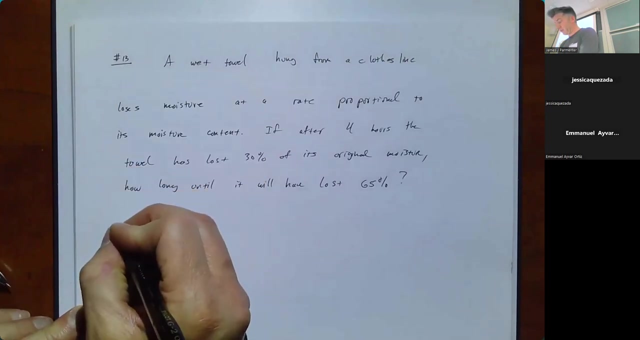 How long until it will have lost 65%? We're probably not actually going to finish this problem, but we are going to definitely do the setup and talk about what we're doing. So before we answer this question, we have to actually find. 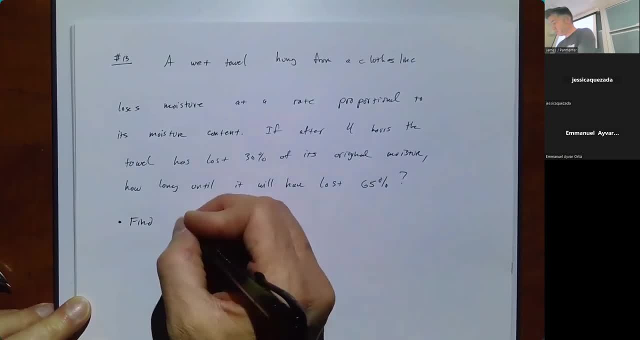 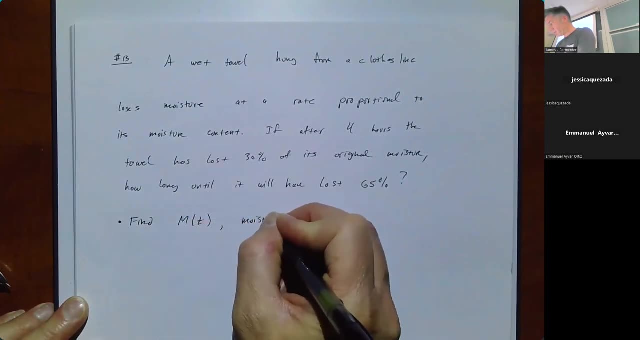 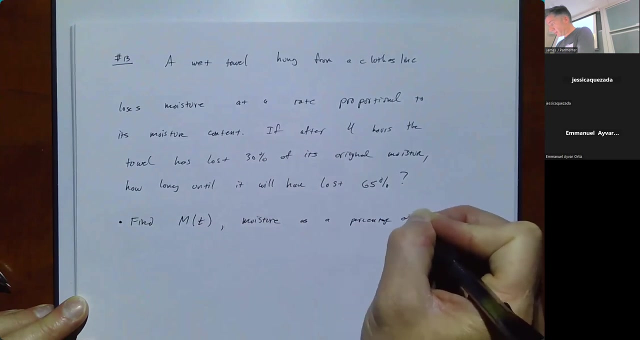 Let's call it M of T for the moisture at time T, Unless they know, they've not given me Moisture as a percentage At time T. We have a couple of, So here's what we're given. We are given. 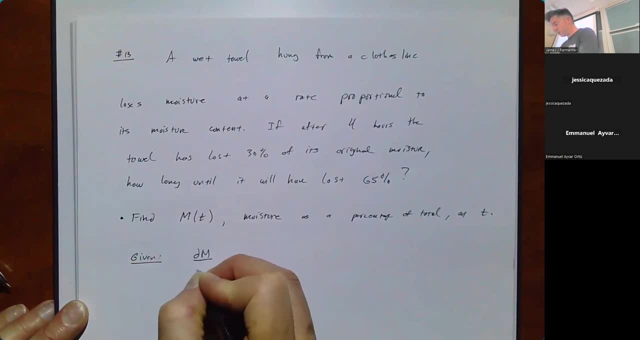 That the rate of change of moisture D, M, D, T or D, whatever, D T right? The rate of change of everything is always D that thing over D T. We're told that it's proportional to the moisture content. So that's just going to be some constant times. 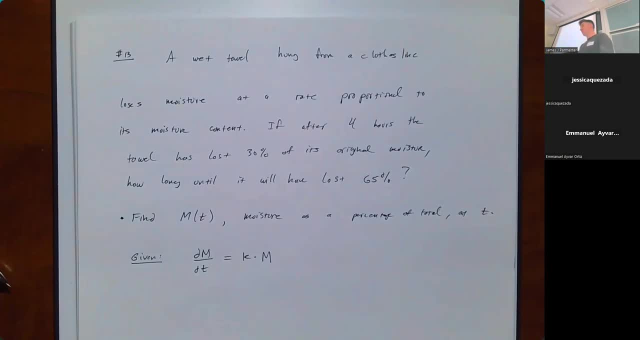 The amount Moisture. This is a pretty standard differential equation. You might have seen this enough that you just, like you, know what the solution looks like. I will, In fact. yeah, I think it's worth. So this one's, we're probably going to solve it because it's not too terrible. 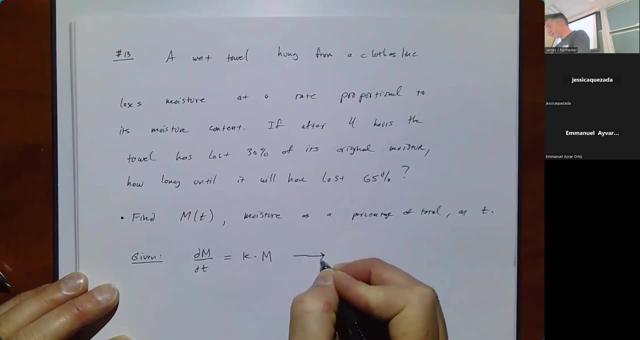 I'll point out that when you have this specific situation, you're automatically going to end up with M of T equal to C, E to the K T. That is the standard, typical solution for when the rate of change of something is a multiple of. 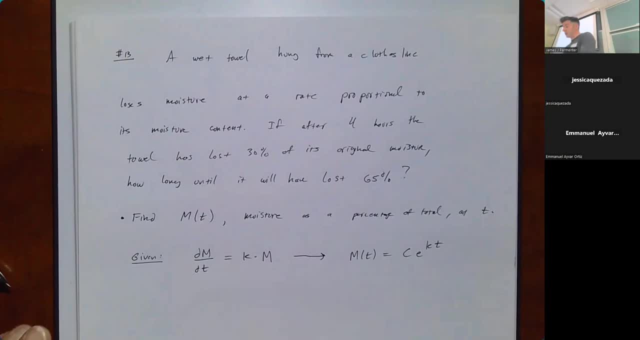 That same something. You could also solve it, though, right. We could definitely solve this by saying one over M D: M is equal to K D T, integrating both sides And getting the natural log of M equal to K T plus C, and then exponentially both sides, and getting M equal to E to the K T plus C, which then becomes. 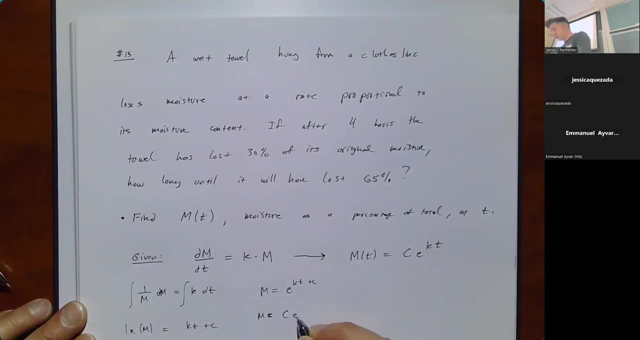 E to the C times, E to the K T, Which is just a new constant E to the K T. So it really is the same. Yeah, I said we weren't going to solve. I'm totally, I'm totally going to solve it right. 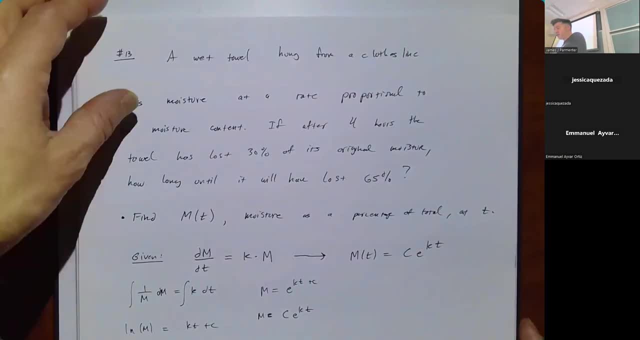 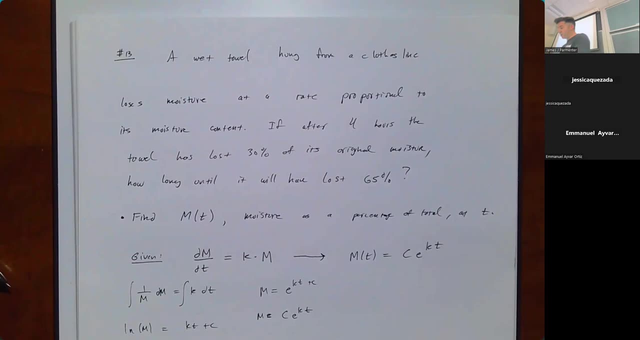 Because there's something, there isn't something I think that's worth mentioning. So we're given a couple of initial conditions. We're given well, we're given one of them explicitly and the other one is kind of implied. So we know. 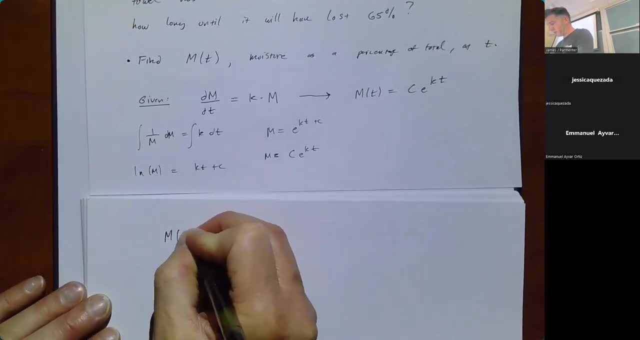 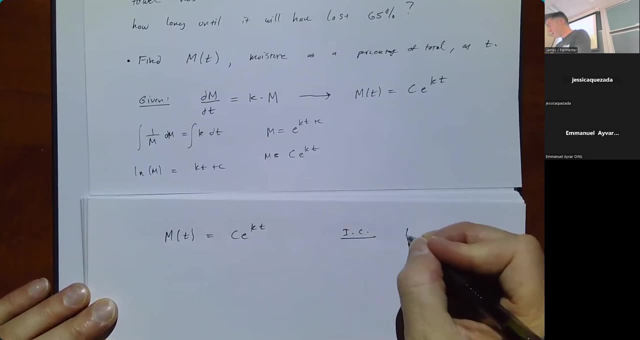 So we've got the following: We know that M of T Equals C E to the K T, and here are some initial conditions. We know that, at time equal to four hours after we observed it, the amount of moisture that's been lost is 30%. 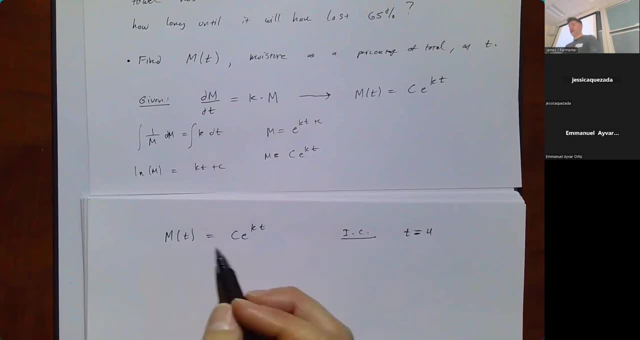 Okay, but that's not what this says. This isn't telling us how much moisture we've lost. It's telling us how much- how much moisture we have. So after four hours, the amount of moisture remaining Should be 70% of the initial. 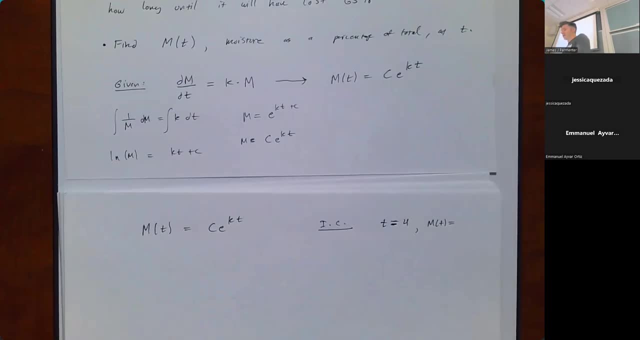 So that's where things get kind of weird. Yeah, how am I going to write this? There's a couple ways you could go here. My preference is typically to say in the beginning: I like to pick an amount, I'm starting with. 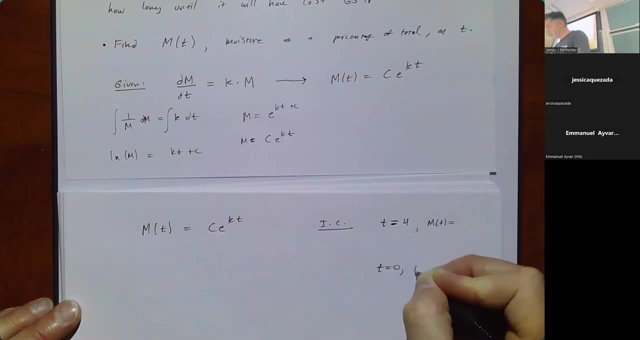 I would personally choose to say that time equals zero. M of zero is a hundred, Probably like a hundred percent. I guess percent might make more sense here, because we were thinking about: right, it's a hundred percent moist, You wouldn't really say it's got a hundred moisture units. 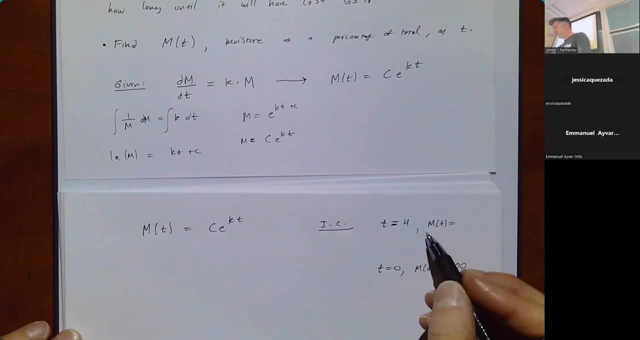 But whatever. So then four hours later, if it's lost 30% of its original moisture, it still retains 70% of its original moisture. Just make sure that when you're writing things down here, you're always writing things down in the terms of how much stuff we have, not how much stuff we've lost. 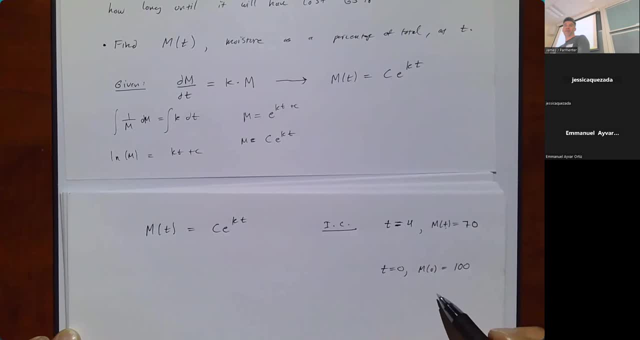 So these are our two initials. This is the one that I was kind of trying to say is implied that we don't explicitly say we start off with a hundred percent. We just kind of know that, oh yeah, we're starting off. 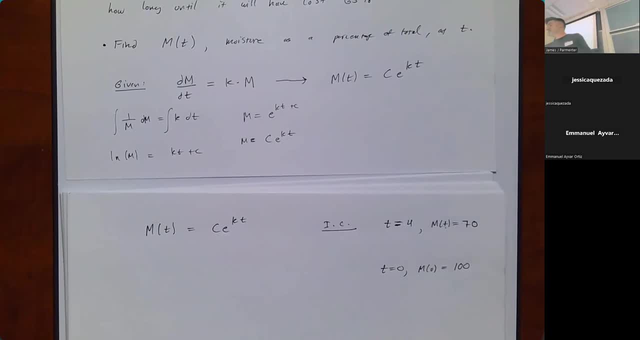 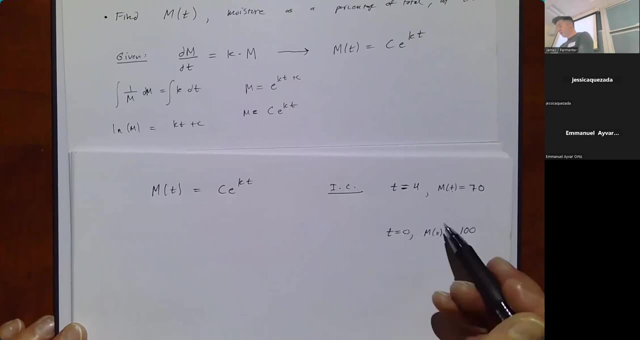 At the beginning, observation with a hundred percent of the moisture that's observed, And then the rest. of this is not too terrible, You would. I would start here and say that M of zero is C. e to the K times zero, which is equal to a hundred. 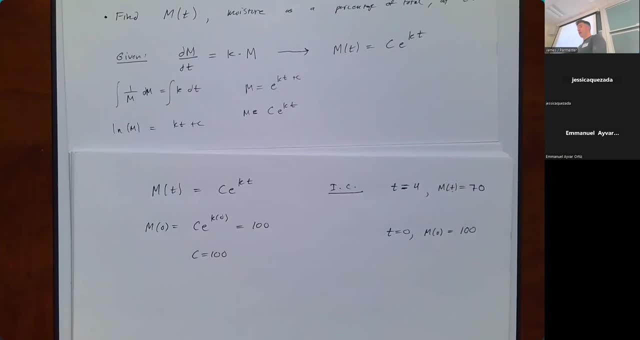 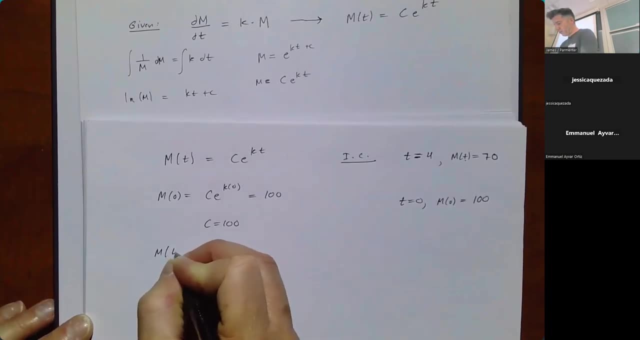 You're going to end up getting C equal to a hundred, And you can write percent if you want to. I think we don't need it, We can just know what it means percent. And then M of four is equal To see. oh, but C is a hundred e to the K times four, and that's equal to the percentage of moisture remaining. 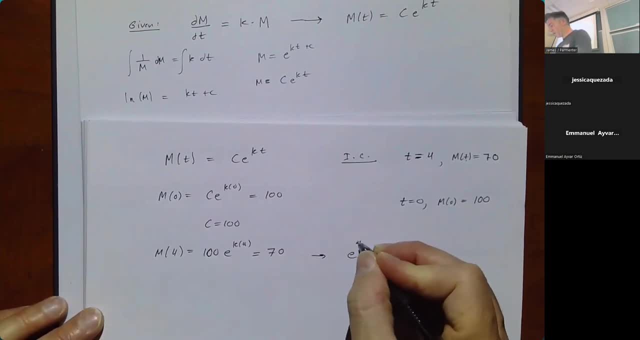 And then we can find K. you get e to the four K equal to 70 over a hundred, which is 0.7.. So then four K is equal to the natural log of 0.7.. So then K is equal to one fourth, the natural log of 0.7.. 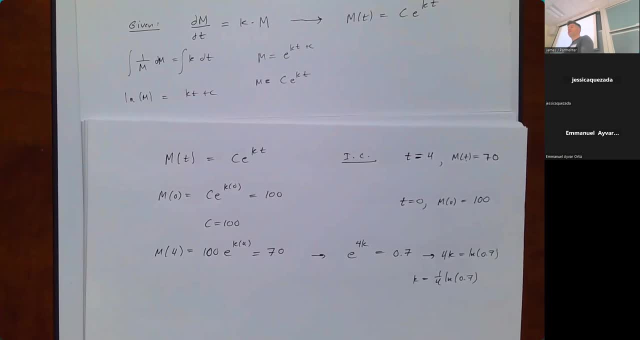 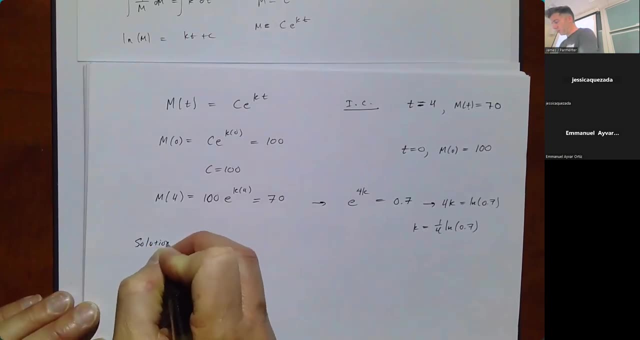 So then you've got the model, and I'll say usually so, the model AKA the solution. that's often what we're looking for. So the solution slash model is that M of T is equal to a hundred, e to the one fourth natural log of 0.7 times T. 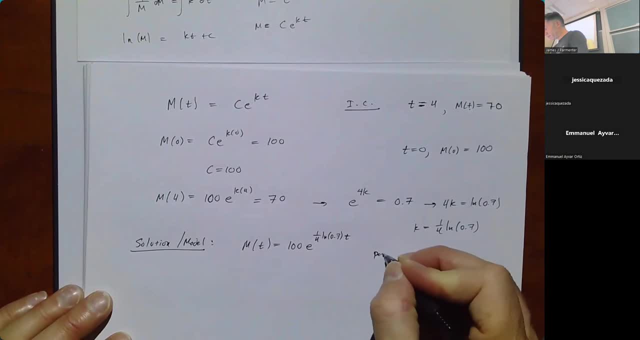 I guess I can say percent. So if T is zero, we've got a hundred percent of the moisture, And as time goes on we have less and less percentage of the original moisture. And then, lastly, if we wanted to solve the question that was asked, which is how long until we have lost 65%- be careful here. 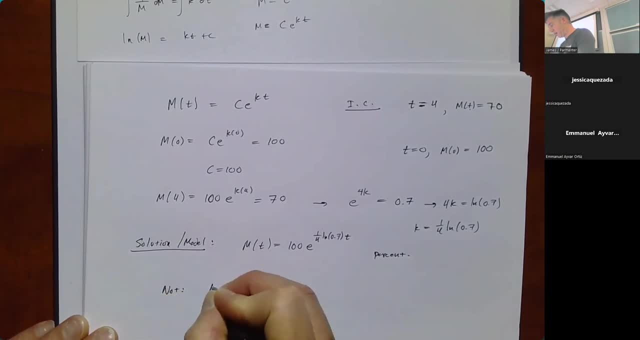 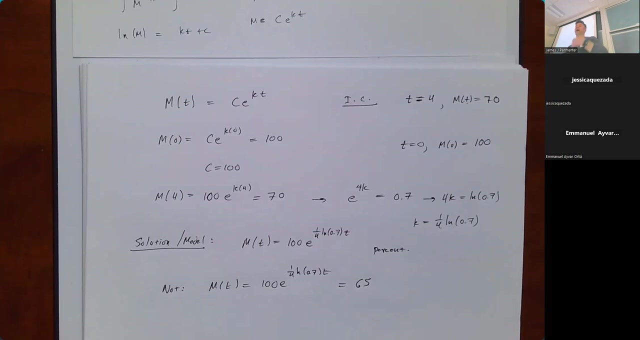 We don't want to do this. We don't want to set M of T, which is a hundred e, to the one fourth natural log of 0.7 T, equal to 65. Because we're asking how long, How long it takes until you've lost 65%, which means one, how long until we have remaining 35%. 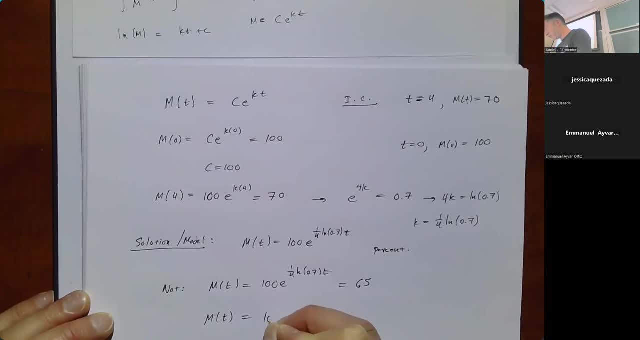 So sometimes problems like this try to be, I would say, kind of tricky with the language that they're using. Make sure you're always thinking about how we want to be talking about how much stuff we have, not how much stuff we have lost. 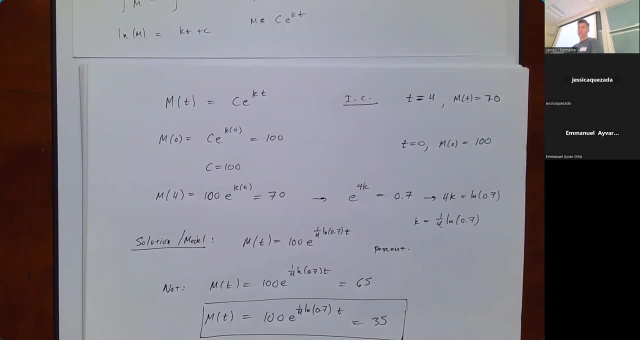 Questions on either of these. Let's try and do one more word problem, but we'll really actually just do the setup, Maybe, And then we'll talk more about some 3D graphing stuff, because that's definitely what we're moving. 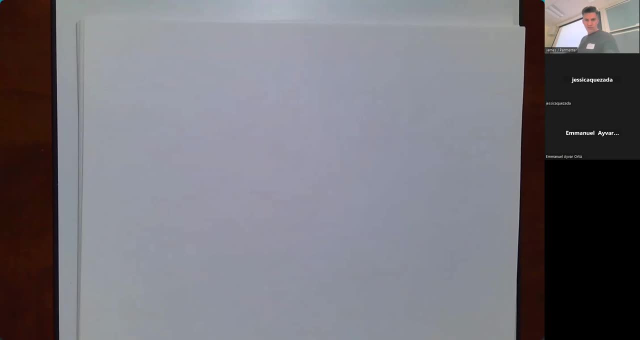 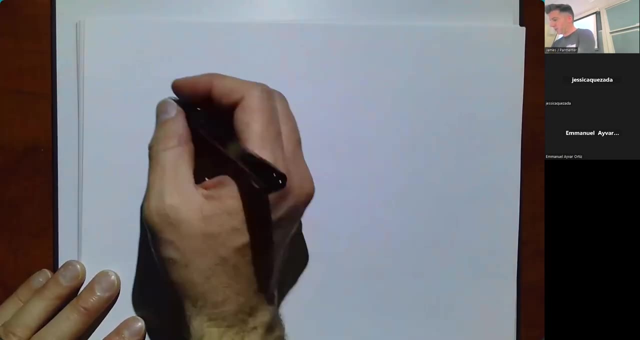 We have moved towards, but people were asking about: let's see, let's make sure. Yeah, People were like: let's see some more problems, Okay, So let's see here. Yeah, I like this one as well. This is similar to number eight. 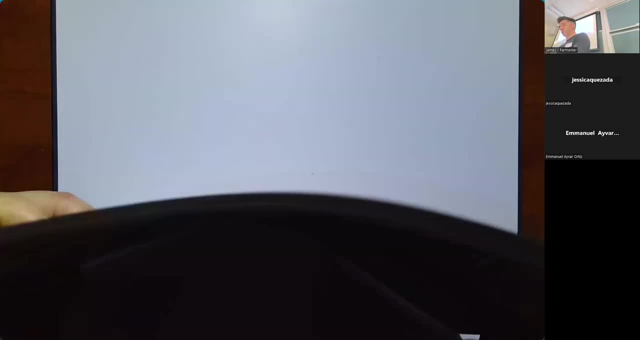 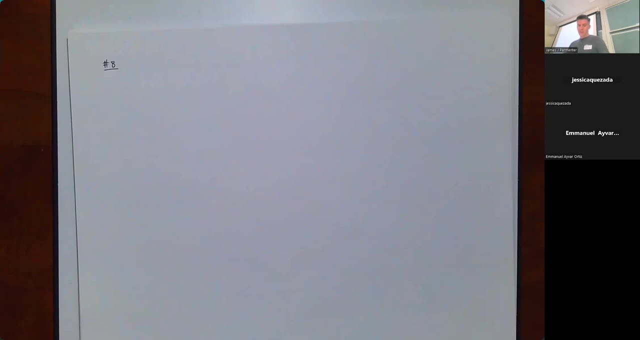 So during a chemical- and I'm just going to- so here's what I'm going to say- I'm going to read the words of this problem and then we'll write down what I think is important. So during a chemical reaction, substance A is converted into substance B at a rate that is proportional to the square of the amount of A. 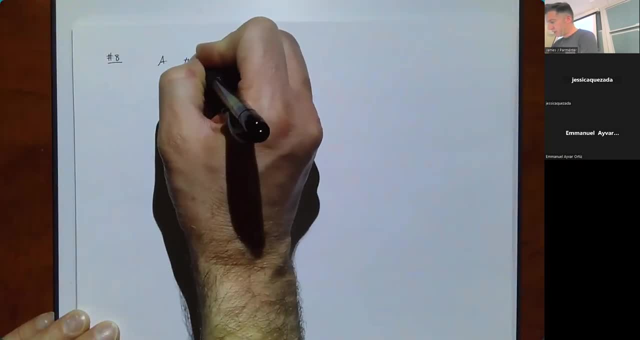 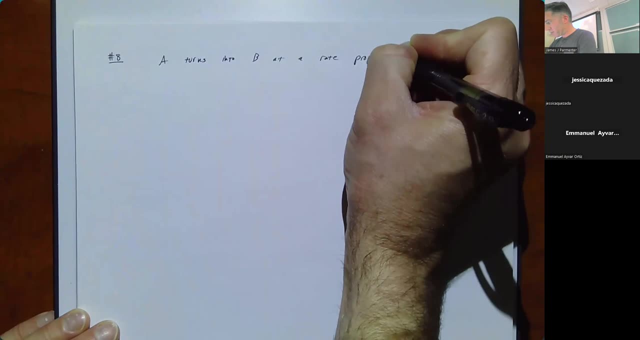 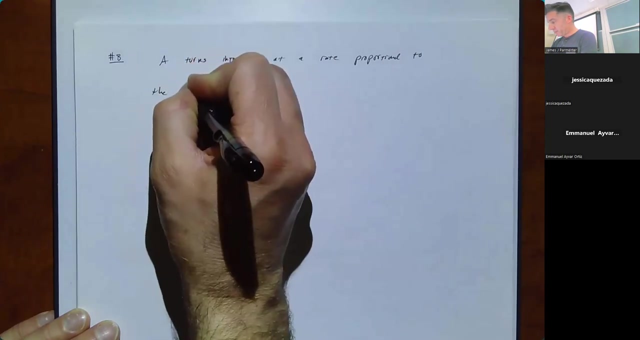 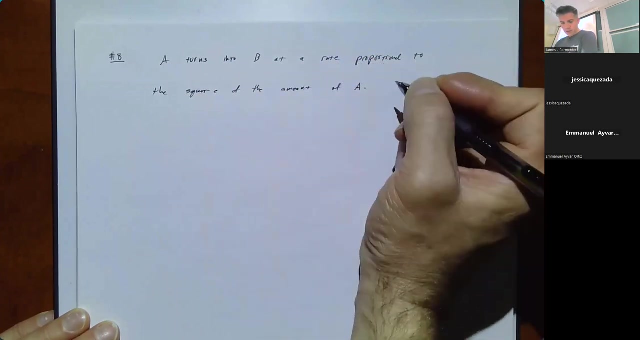 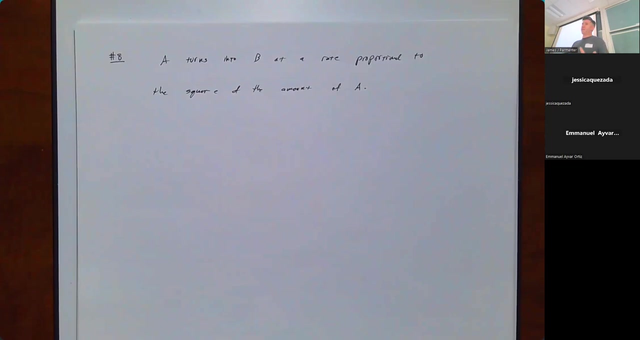 So I'm going to write down: A turns into B at a rate proportional To the square of the amount of A. So to me it looks like I feel like this B part really isn't super important. Like they're saying, A turns into B, but really we're just caring about the rate of change of A. 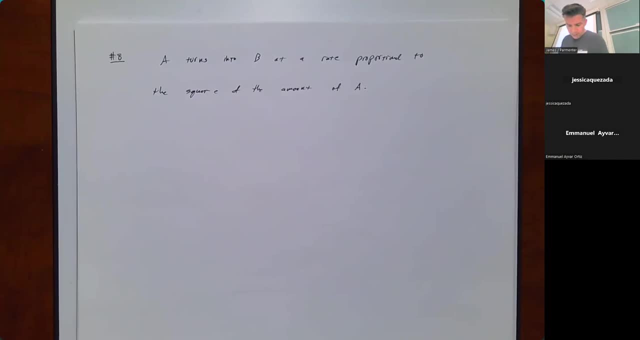 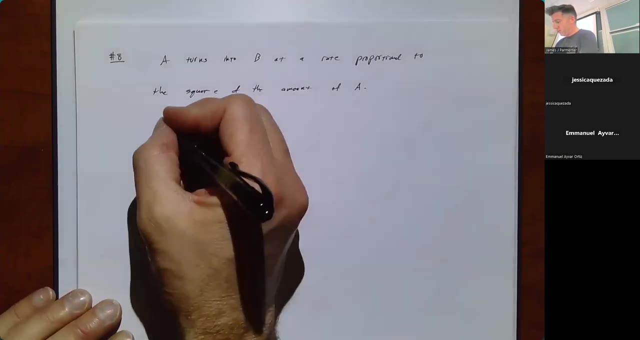 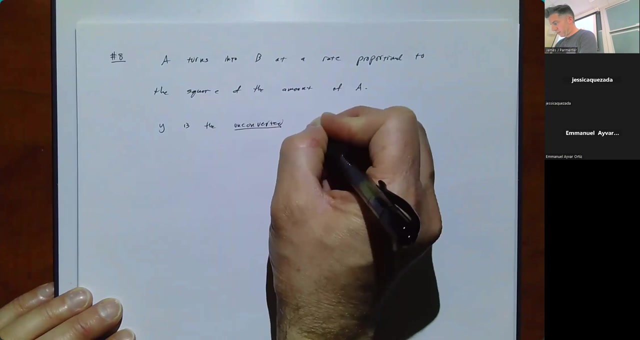 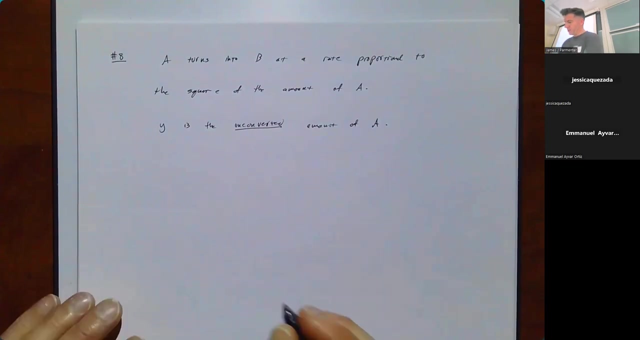 Let's read the more of the question before we fully decide on that. Let Y be the unconverted amount of substance A at any time. T, Okay, Y is the unconverted amount of A. Annoying When time equals zero and then they're just giving us some distributions. 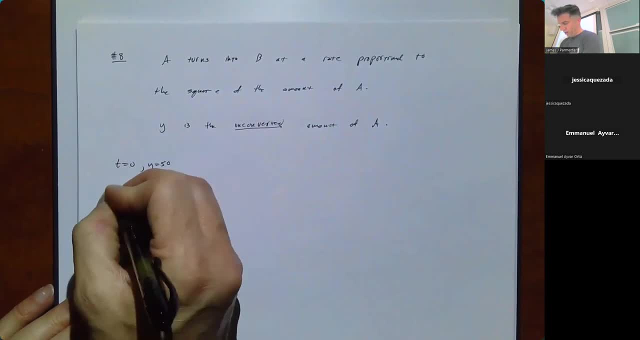 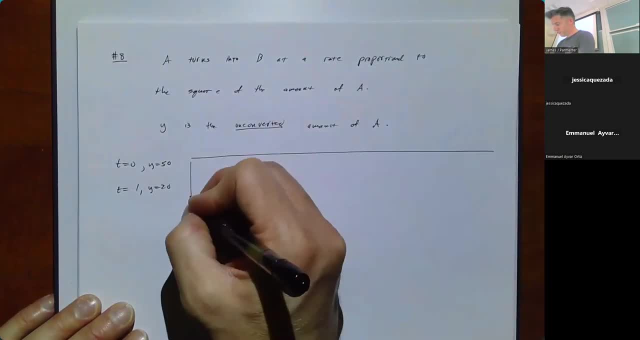 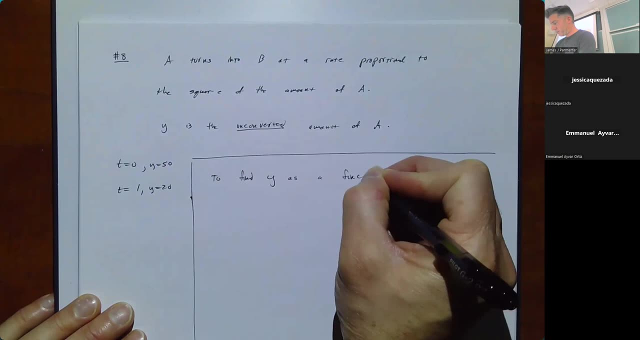 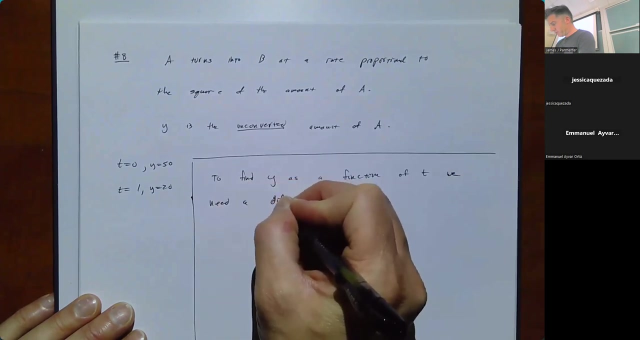 So to find Y as a function of T, we need a differential equation. Okay, All right. So, yeah, What's why? Well, it's the amount of A that isn't converted, right? So how are we going to write that down? Good question, And I'm really asking because I'm 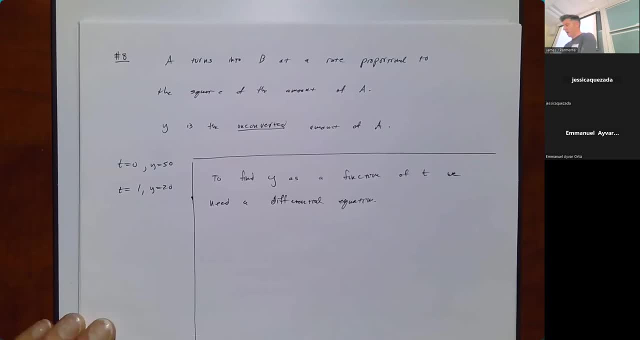 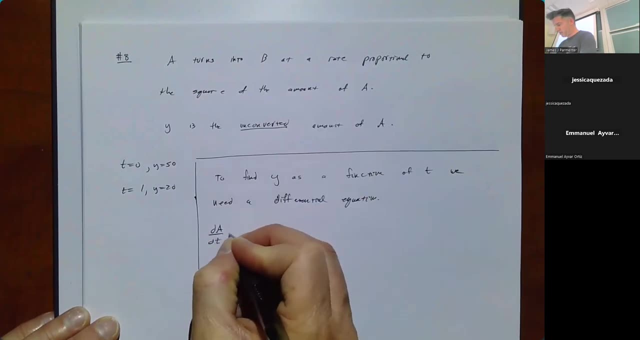 just thinking about. what are we really doing here? Here's what I'm thinking about. I know that the rate of change of A and the ADT is equal to some constant times the square of the amount of A. That might be helpful. It might not. Why is the unconverted amount of A? So I guess Y is. 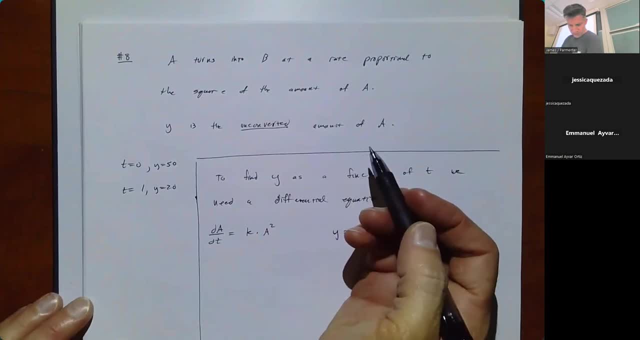 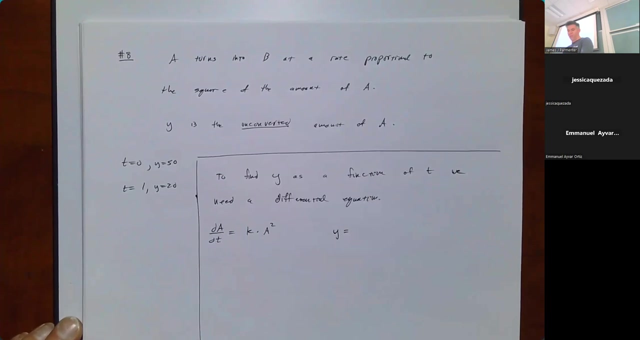 equal to. I don't love the way they phrase this. Yeah, Good question. Yeah, maybe I don't really. I honestly don't really know. Right, It's kind of funky. So what I'm thinking is that I know that time equals zero, Y equals 50. And the amount? 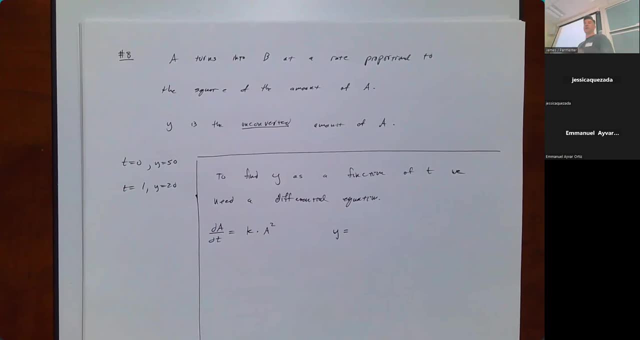 of A that has been converted into B is zero. So to me it feels like A and B have to add up to 50. Right, Does that seem plausible? I think so, Because we're going to write that down, Because we're starting off with 50. And they don't say that we're losing stuff, We're just 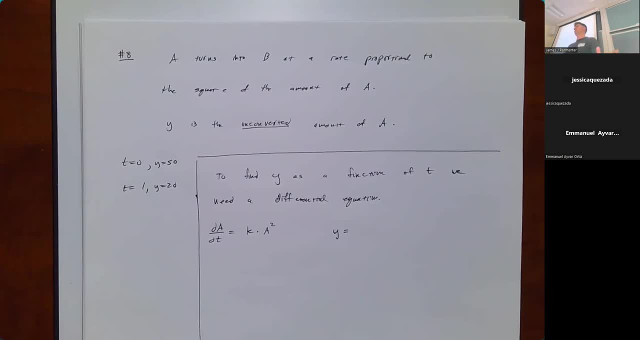 saying one of them turns into the other. I feel like in these problems sometimes there's a lot of chemistry, kind of assumptions in the background that aren't really getting fully explained or thought about. We're just going to say, yeah, this thing turns into that, We're not losing. 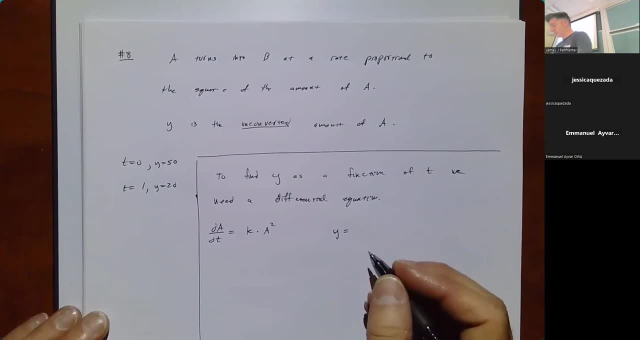 anything, We're not gaining anything. So I think we should be saying something like: well, we know that A plus B equals 50. But yeah, why? So I feel like, what do I feel like? I feel like it's kind of funky. 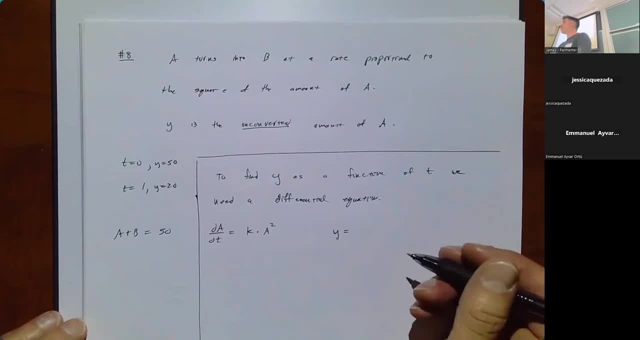 But it's still being. do you think it's because, like I'm increasing it? Right, As time increases, Y is going to decrease, Right? So I think what. I think what we want to do, and I'm not 100% sure, but the way I'm imagining this, I think we want to think of Y as 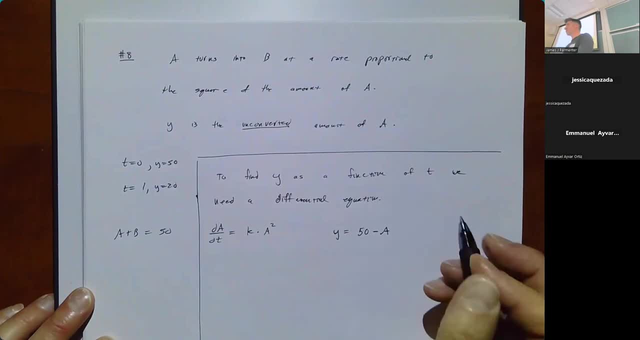 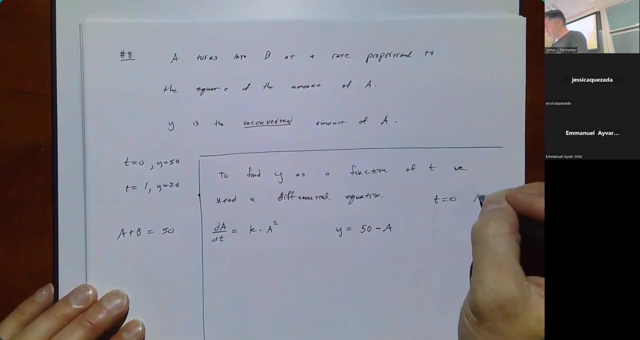 being 50 minus A. Here's why A time equals zero. So when time equals zero, A equals zero, Y equals 50. That seems reasonable, right? And then the equation we're going to write down is that? well, I think I can say A equals 50 minus. 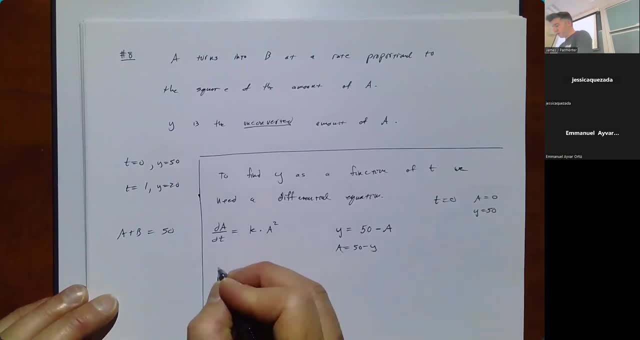 Y. So really I want the rate of change of 50 minus Y to equal the rate of change, sorry, to equal 50 minus Y. So I'm going to write down. well, I think I can say: A equals 50 minus Y. 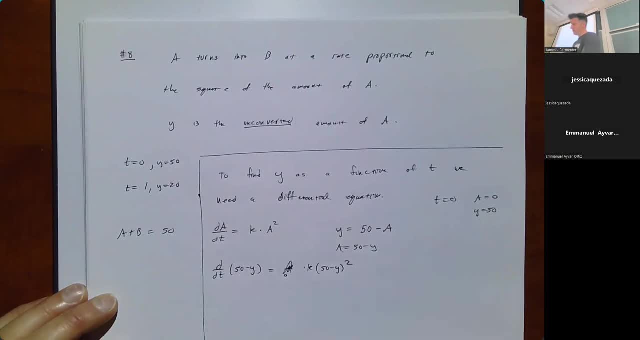 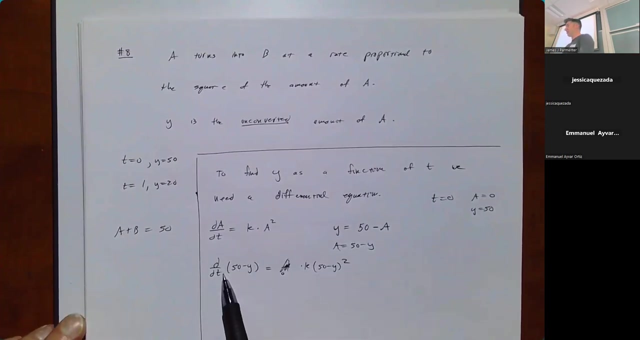 Okay Times 50 minus Y squared. It feels funky. I feel like I'm leading you astray, to be perfectly honest. So good question. Setting these up is hard, right, Like it's not always super easy to identify what's happening. I feel like this: I feel dicey about this, to be very 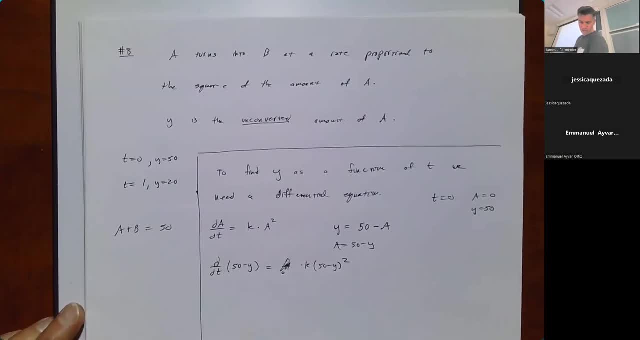 honest. Yeah, I don't like this question. I looked at this one and I was like maybe, And then I was like I should have just avoided it, But I didn't. so Right, Why is the unconverted amount? So we know that the rate of change of A is proportional to how. 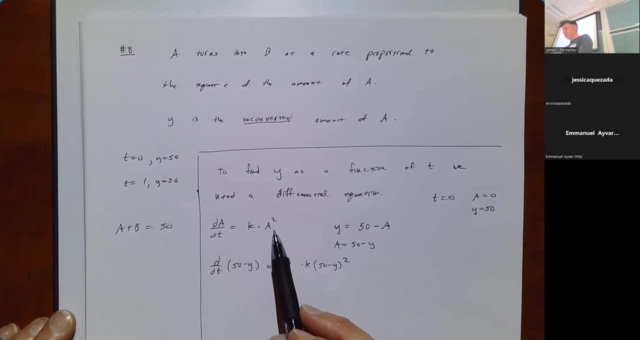 much A squared, So it should be that I feel like this is fine. Yeah, I don't. I don't feel like this is wrong. I feel like the rate of change of 50 minus Y, which is just what A is the amount. 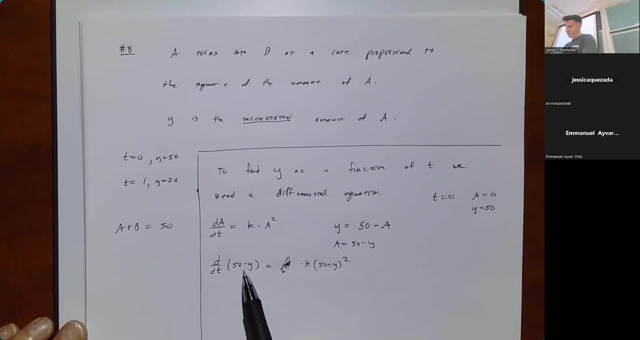 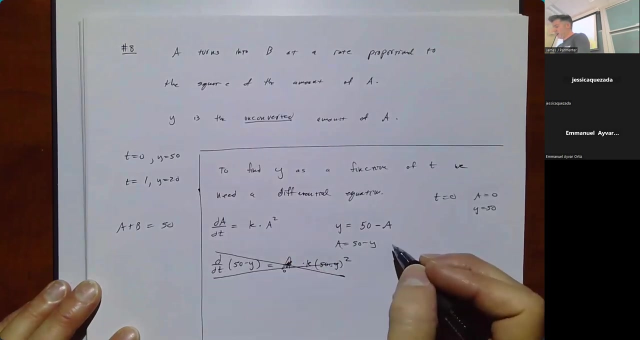 that hasn't been the amount that. Would you just sum it to 58?? Maybe, Yeah, that's probably. yeah, I like that idea better. That's a. that's a good idea, So let's scratch this. Yeah, I think, I think you got the right idea, So we can definitely solve. 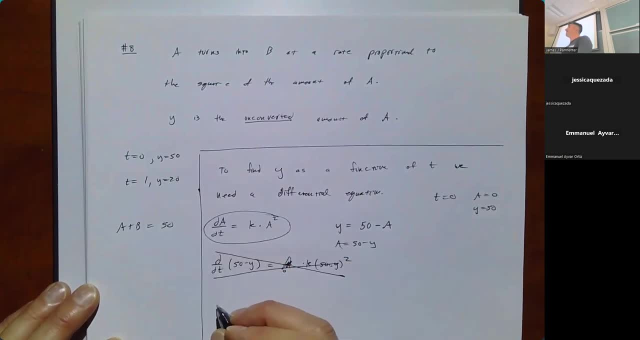 this, which is not too bad. We can say that I know all right, so we're just going to set it up once again, not just setting it up. We have that 1 over A squared times DA is equal to K times DT. 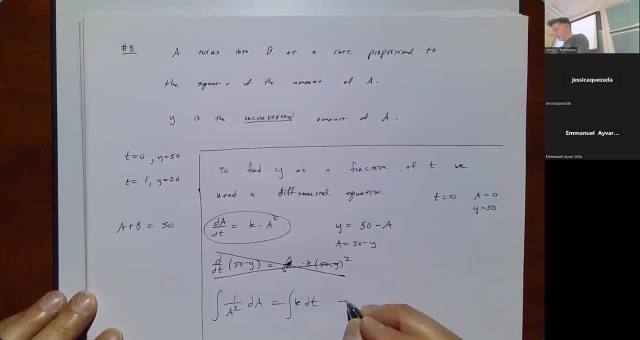 I feel like we see 1 over A squared, enough that you should get used to seeing that. oh, we know that the antiderivative of 1 over A squared is negative: 1 over A. And on the right-hand side again, we. 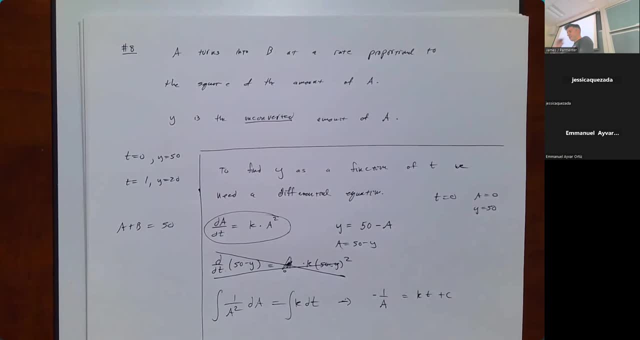 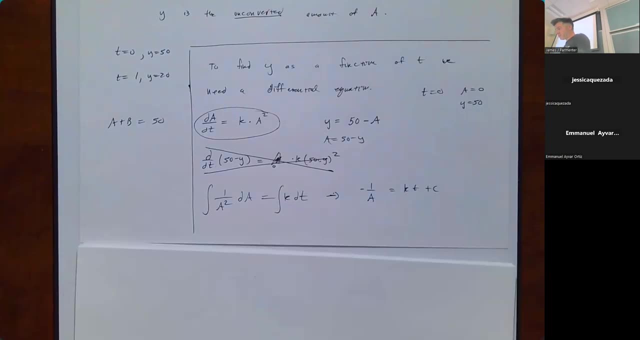 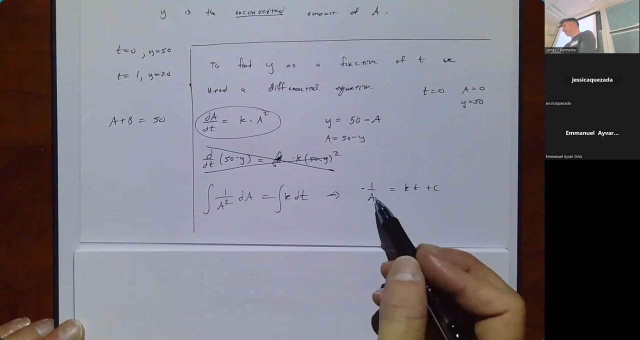 have a KT plus C, So then we can solve for A Here's. so watch this real quick. I'm going to multiply both sides by negative 1.. I think in class she actually does multiply both sides by negative 1.. You can get away with not doing that, but let's go ahead and do it that way. 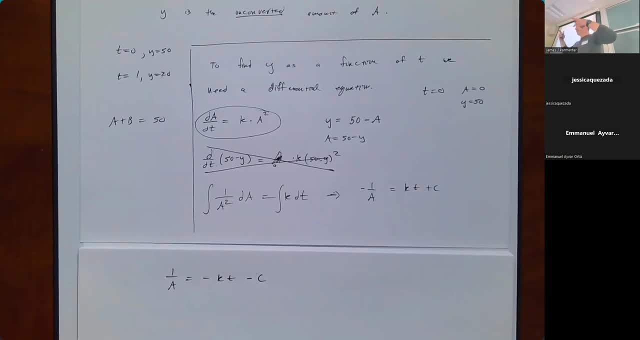 So 1 over A is equal to negative KT minus C, And then we take the reciprocal of those sides So that the A as a function of T is equal to 1 over negative KT minus C. And I think what we say is: A is 50 minus Y. 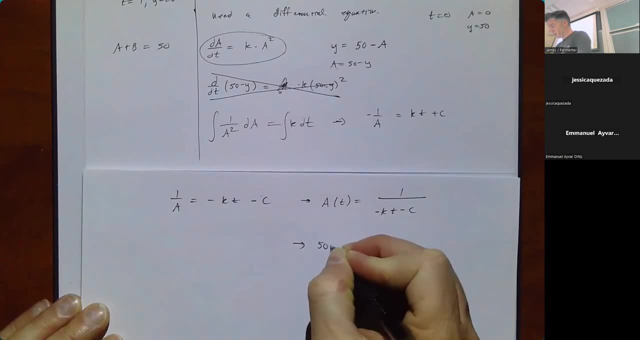 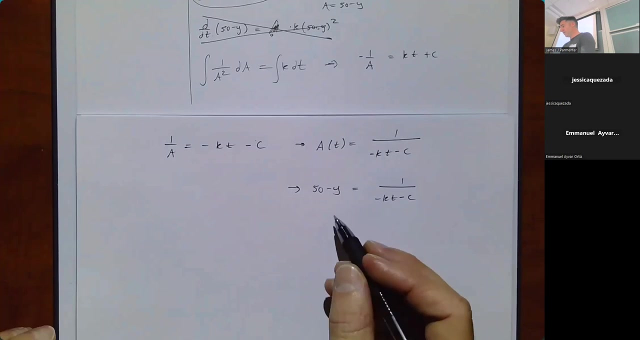 So we could just replace this with: 50 minus Y equals 1 over negative KT minus C. Yeah, that seems a little strange, though. I mean strange, not wrong, just strange. And if you want to solve for Y here, we can say that Y is equal to. I'm going to just think about. 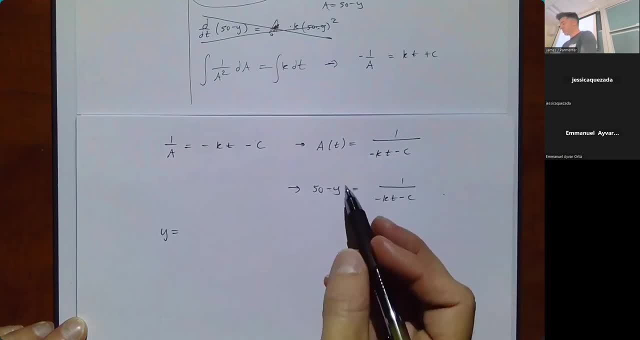 adding Y to the right side and subtracting this over here. So Y is equal to 1 over positive Y, And then we can just replace this with: 50 minus Y equals 1 over negative KT minus C. So here we go. 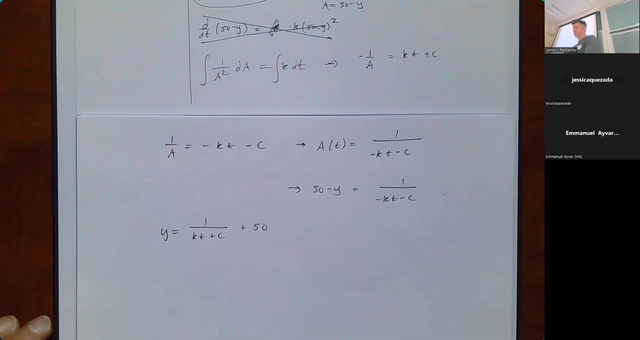 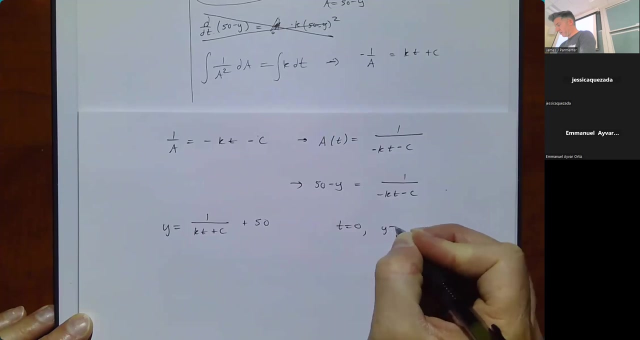 Y is equal to negative KT plus C plus 50.. Seems interesting. Let's see what we might as well. we've gone this far. we might as well fix it. So here's what we know. We know that at time equals 0, Y equals 50. 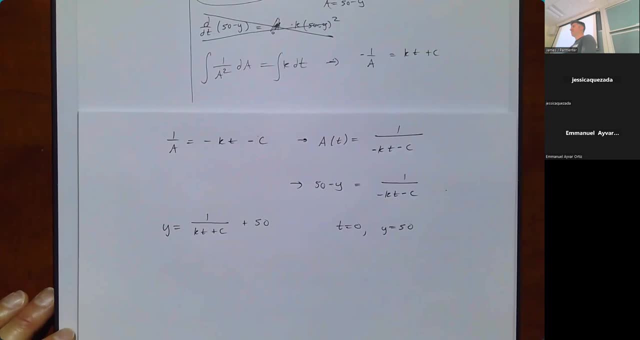 Well, that already seems problematic. Here's why This fraction here is never 0. Which means clearly i've done something incorrectly, right, because this can't with the way we're writing here, which can't be the solution. hmm, hmm, that's a bummer now. i'm not sure. 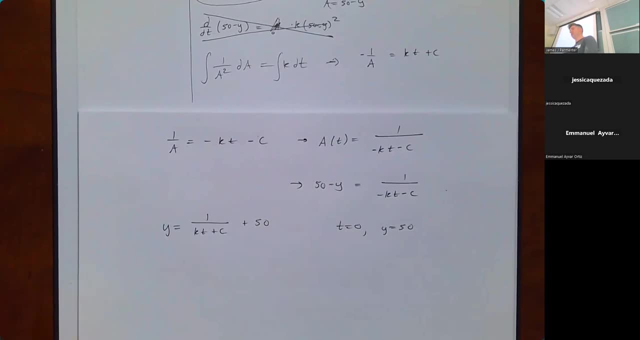 yeah, i think i should think about this one and come back into it, because i i could stand up here and be like, well, let me think about it some more. but really, like, i'm actually not sure. i know i've done this problem before, but i forgot to do it. so i'll think about that. maybe i'll write something. 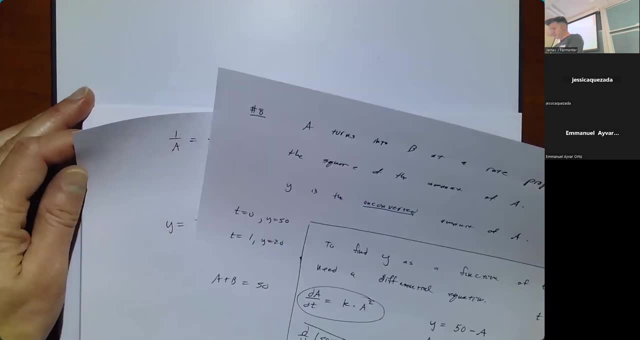 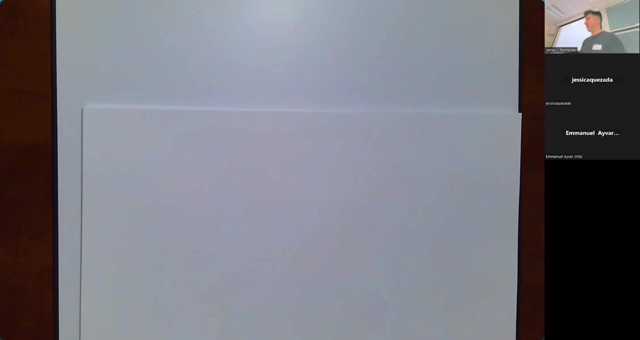 and post it on canvas a little bit later today, because, yeah, i don't remember how this one goes. i'll try not to think about it. okay, let's give ourselves the last 20 minutes of class here to talk about traces, specifically because i think those are important. um, yeah, sorry about that. 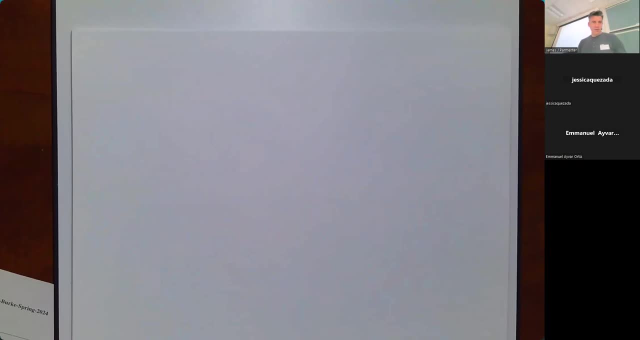 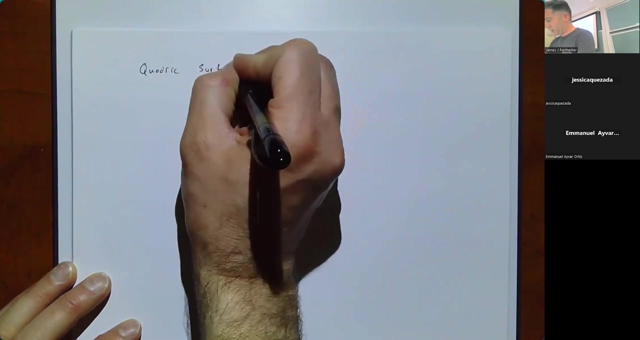 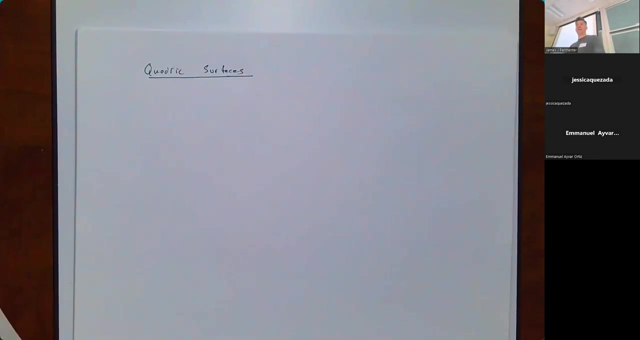 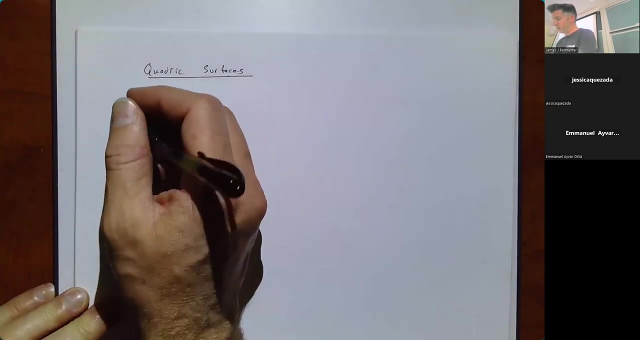 okay, so sketching things, finding traces, let's talk about some equations of quadratic surfaces, which sometimes people mistakenly say is quadratic, but not, it's actually quadratic. um. so there's there's like six of these, and you might have already seen some of them. let me give you an example of one. so let's say we have the following: 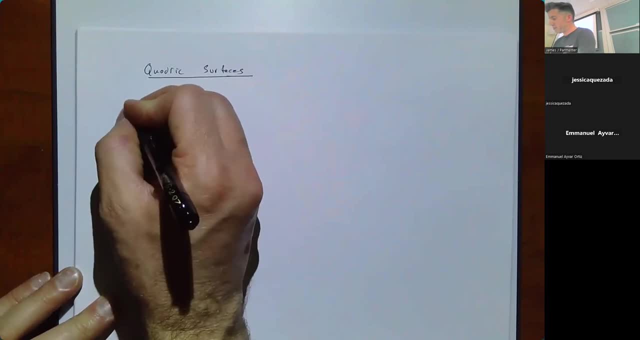 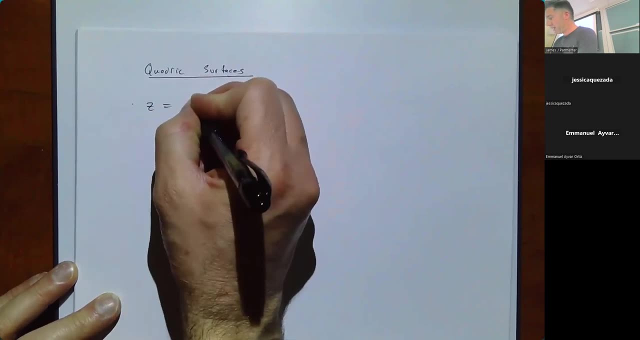 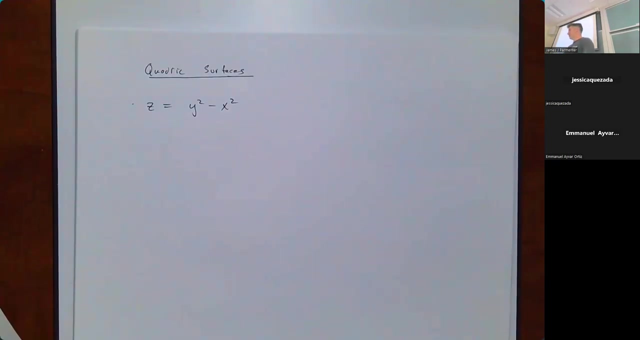 surface? we have sure, let's see we have. sorry, i'm trying to pick which one. yeah, let's do that one, okay. so z equal to y squared minus x squared. so this is an example of one of the quadric surfaces and the way we would usually graph. 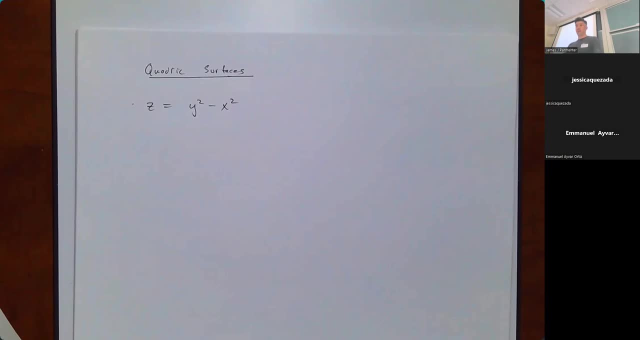 something like this is by drawing the traces in each of the place. so let's draw some traces, so we'll start, and one of the- so sometimes one where one traces is kind of funky. this is that's going to be the case here. let's actually not start with the trace in the xy plane. 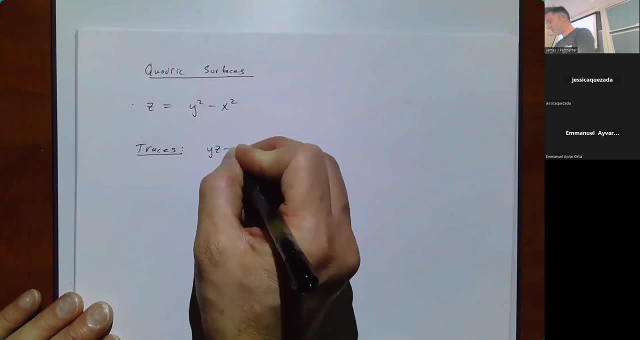 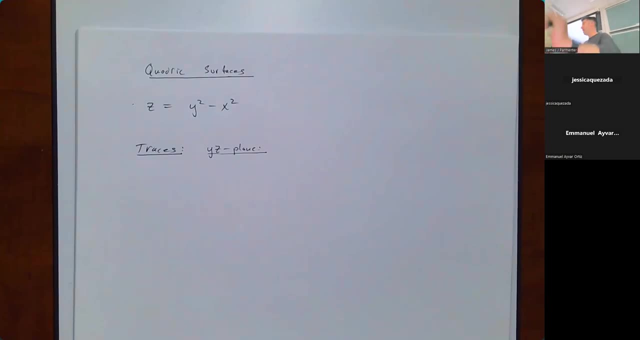 so we start with the trace in the yz plane. if i'm in the yz plane, which i know what's your name, by the way, i knew you weren't here last friday, but i definitely i talked about how, in the classroom, i'm going to think of that corner as the origin and that wall is the y, is the xz plane. 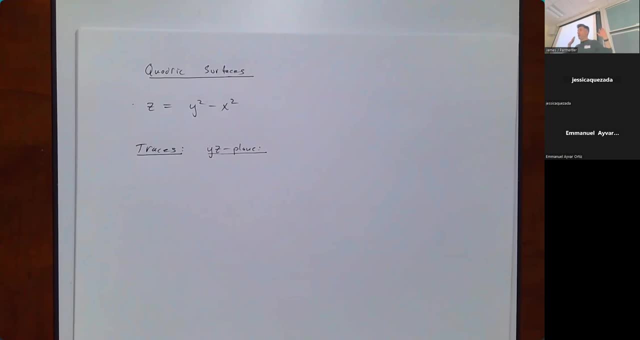 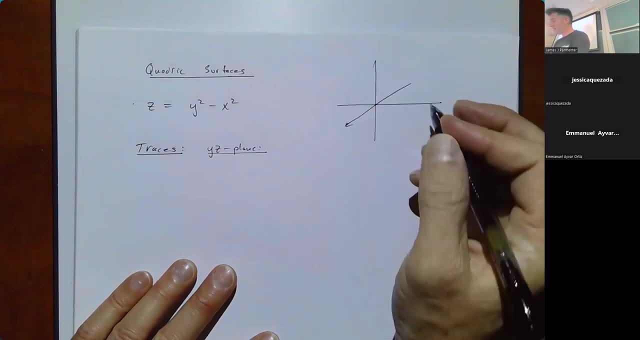 the floor is the xy plane and the wall behind me is the yz plane, which i like, because the yz plane i'm always thinking of as the easiest one to graph in, because the yz plane is the one that's kind of like just flat on the paper. 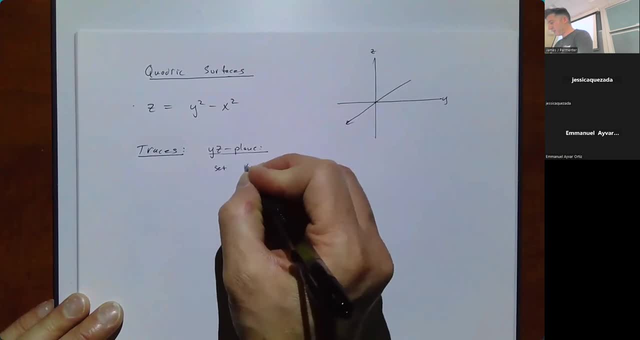 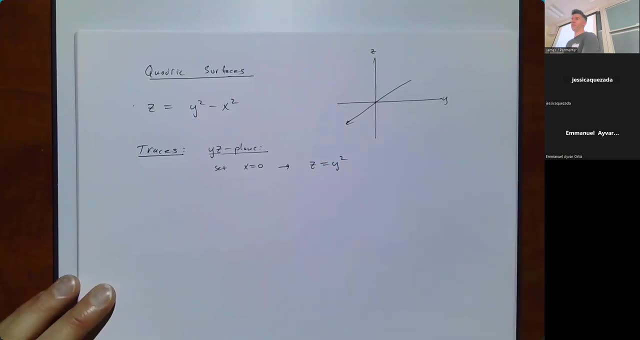 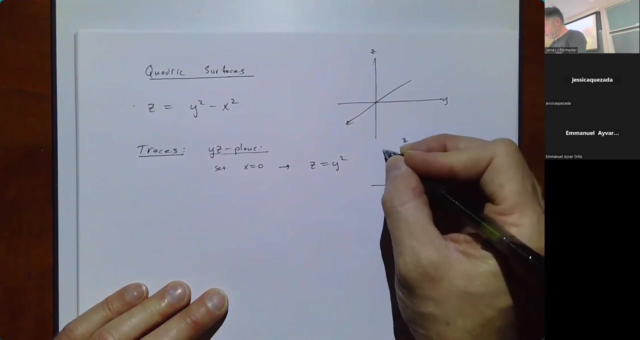 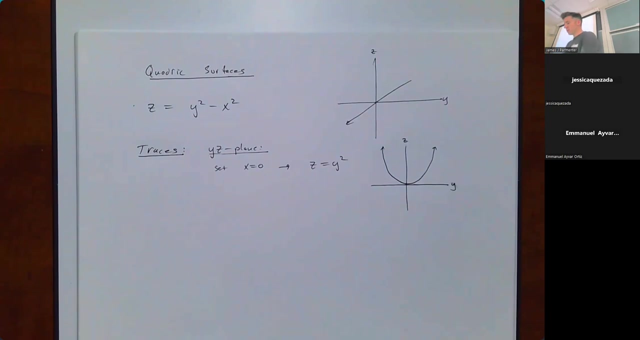 so the yz plane, we're setting the missing variable equal to zero and we're going to get z equal to y squared minus zero, which is just a parabola. so in the yz plane you've got this upward opening and you've got this downward opening parabola whose vertex at the origin 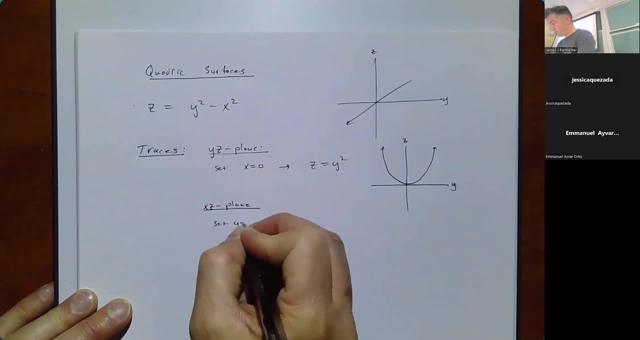 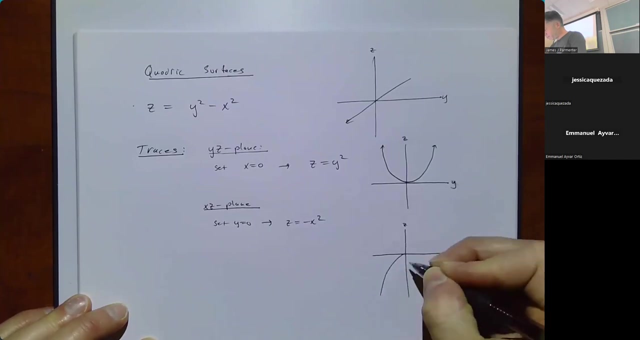 let's look at the xz plane. well, there we're going to set y equal to zero and we're going to get something very sorry. you know what? we have something very similar. we can get z equal to negative, x squared, which is not quite the same, it's just a downward opening parabola. 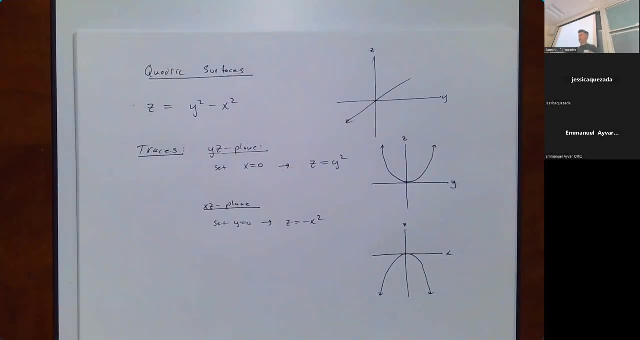 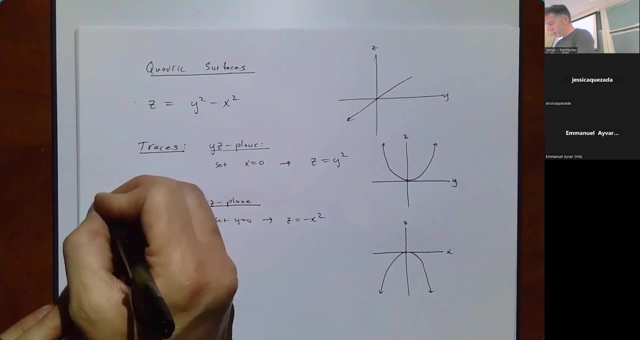 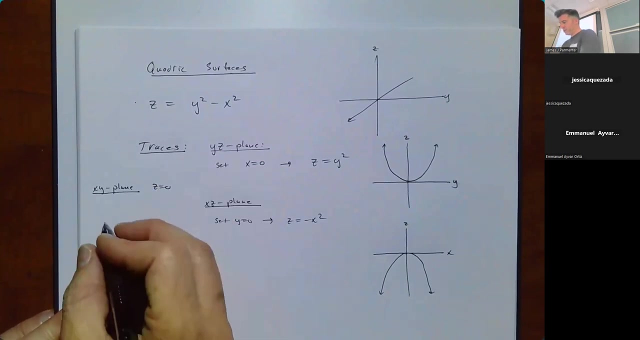 got in that corner over there. i've got an upward parabola going this way and downward parabola going that way and then we should talk about- even though it's kind of annoying- in the x- y plane, when we set z equal to zero, we're going to get zero equal to y squared minus x squared. 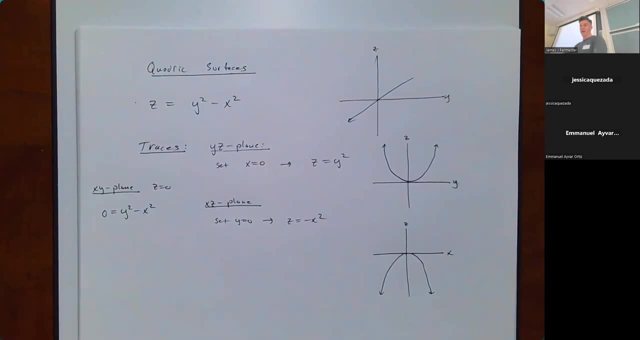 we have to be extra careful here because we get a little bit more than you might think we do. if we bring the x word over to the other side, we get x squared equal to y squared. and if we take the square root of both sides, we don't just get x equal to y, we take the square. 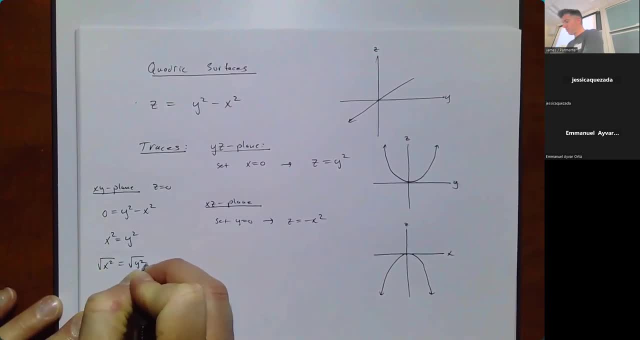 of both sides. well, you might notice that x or y could be positive or negative. y could be three and x could be three, or y could be three and x could be negative. three or x could be three and y could be negative. three or both of them could be negative. right, they can kind of both be any. 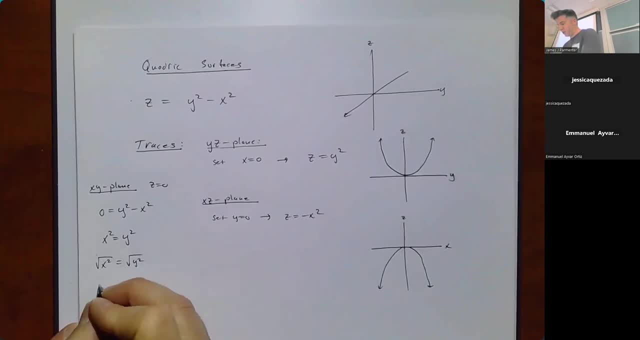 sort of positive or negative of each other. so this equation actually boils down to being the absolute value of x and the absolute value of y, or in other words, y equals x or y equals negative x. so when we graph this- it's kind of weird- you get these two lines. 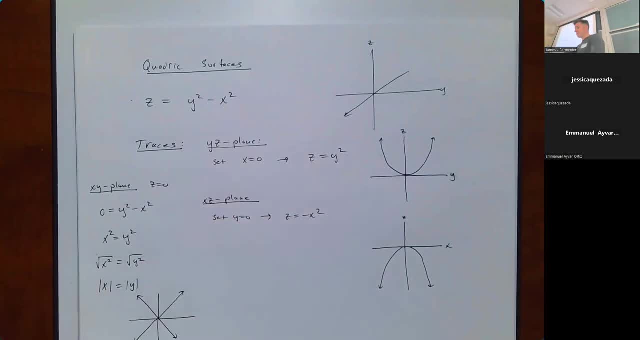 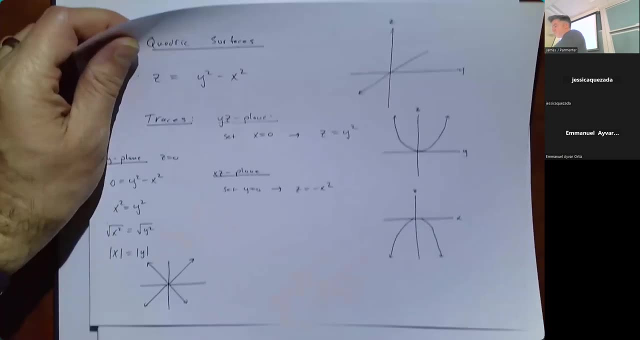 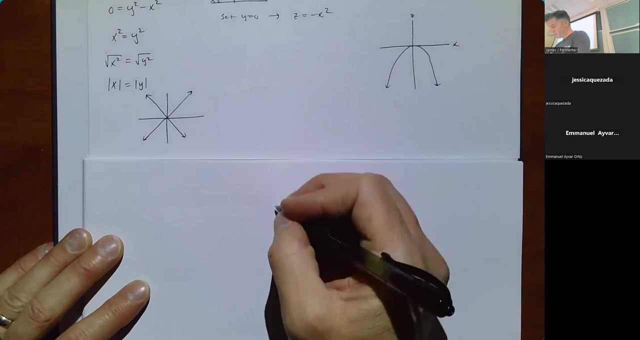 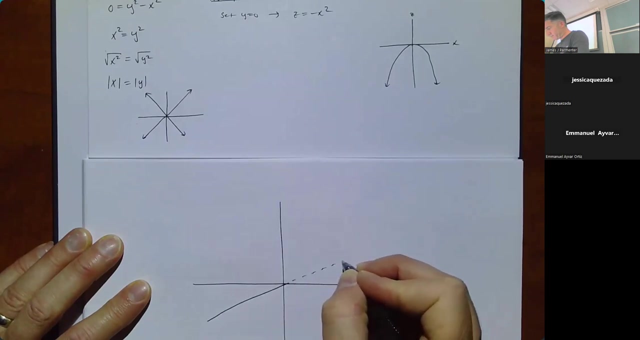 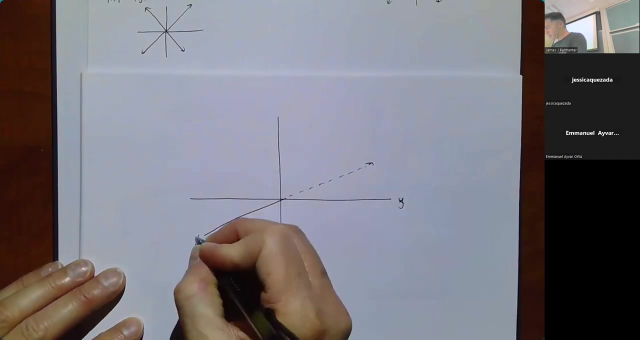 and if we want to try and put it all together, yeah, let's make it big. we're going to put it all together on one big graph, yeah, and we'll talk about some level curves as well. okay, so here is our xyz, xyz coordinate system and i'm going to draw my 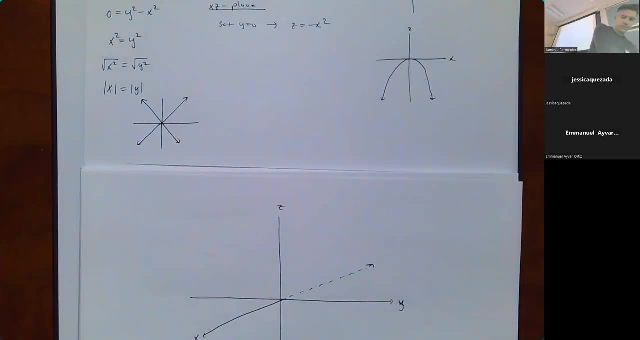 traces and i'm going to draw my traces in each of the appropriate places, so in the yz plane. so i'm i'm always going to try and draw the yz plane first, because and actually i'm not going to draw all my traces, so i should back up for a second. 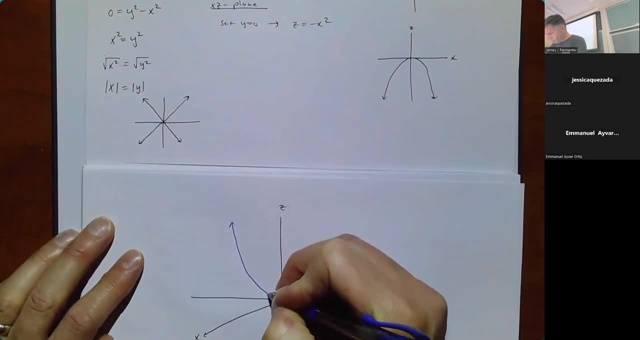 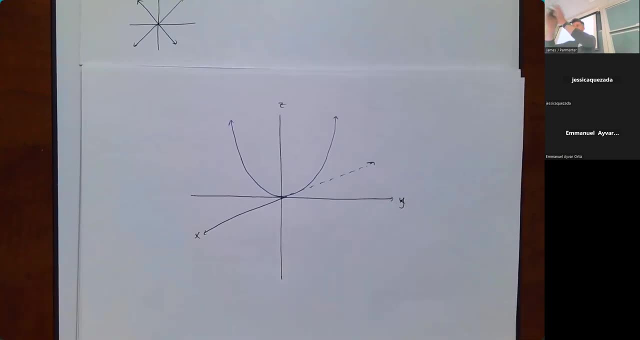 so here's my trace in the yz plane and it's looking parabola there, and then the xz plane, which is the one that's kind of coming out towards you. i've got a downward open problem, so it's going to kind of look like this. it's going to be: 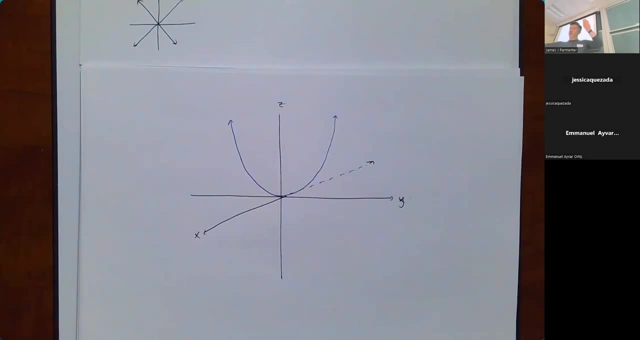 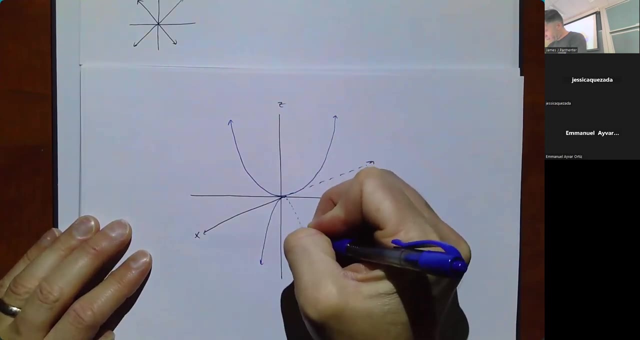 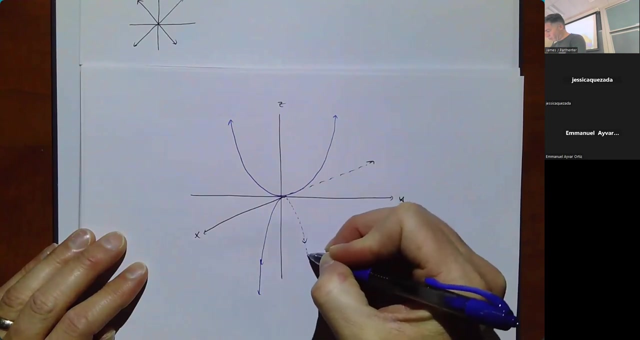 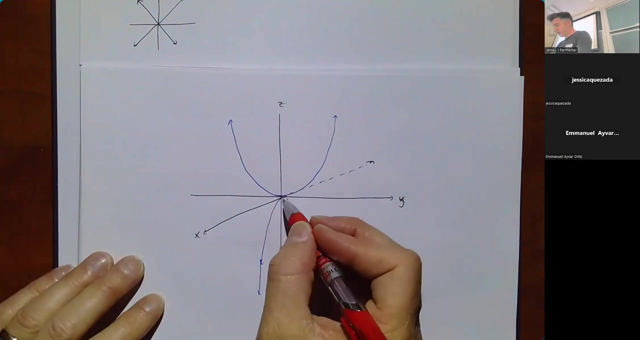 it's not going to be quite as wide. right, i'm taking that parabola and tilting it towards you like that, so it's going to look kind of like this: right, obviously, these things keep going and then in the xy plane i'm not going to draw them, but i would have like. 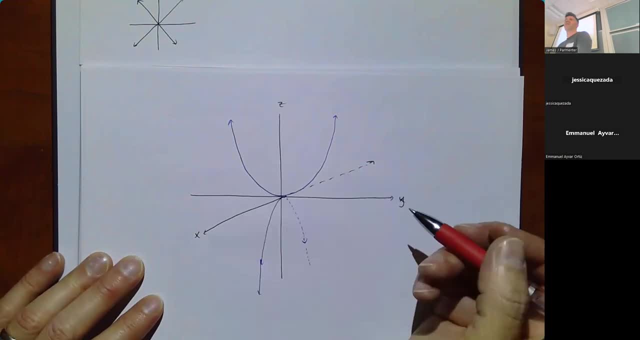 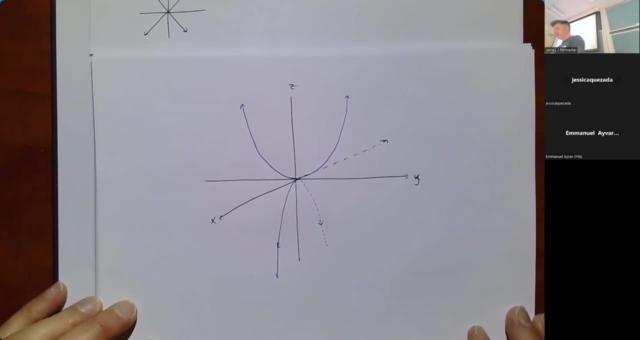 essentially diagonal lines going this way, in that way, which i know is kind of funky. let's draw the rest of the surface and maybe we'll see what's happening here. so actually, I'm going to draw. so I'm going to draw this because I know how to draw it. 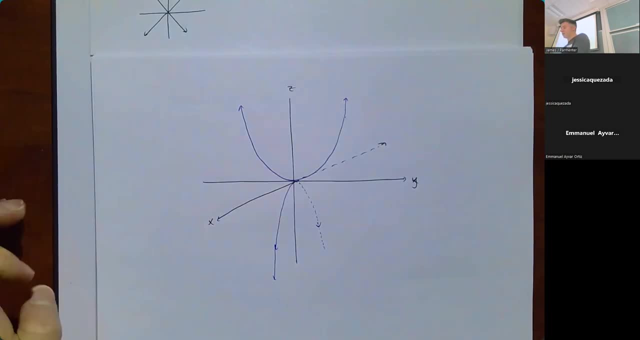 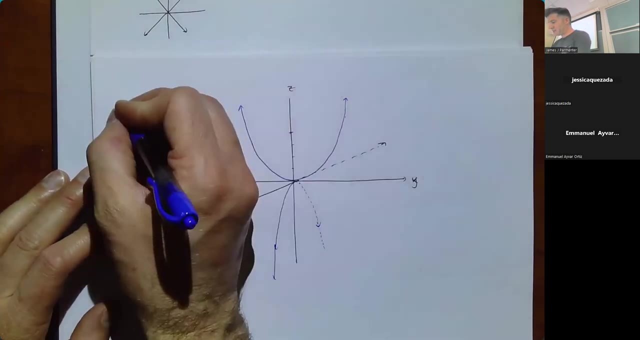 let's talk about the level curve. let's say we went up 1,, 2,, 3, 4. so let's go up 4 units. so let's say we set z equal to 4 for a second. well, if z is equal to 4, 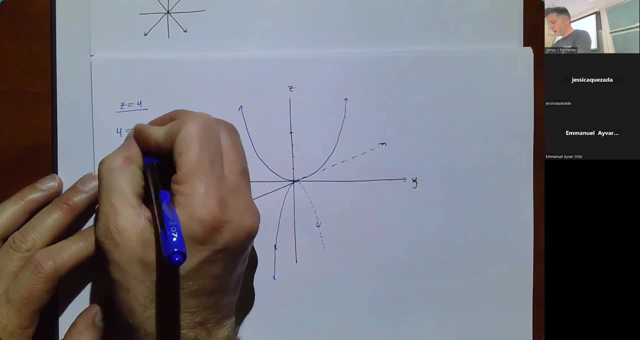 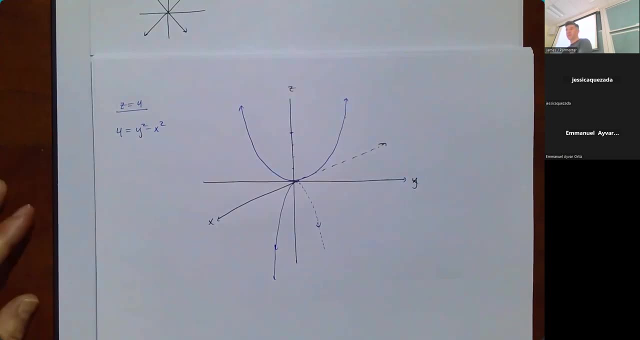 then my equation is going to be 4 equal to y squared minus x squared, which you might not have a lot of experience graphing. when you have something like this, it's very, very close to looking like the equation of a circle if it was just x squared. 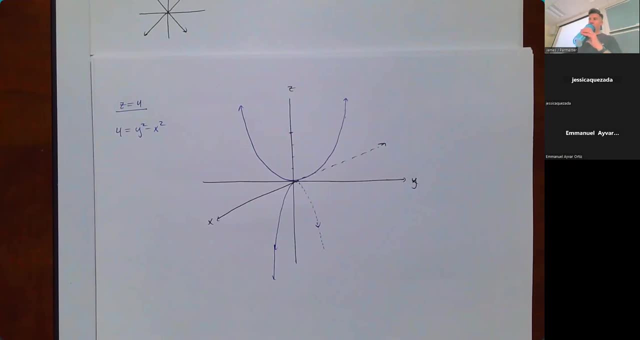 plus y squared equal to 4, we'd have a circle of radius 2. when it's x squared minus y squared, or y squared minus x squared, we have a hyperbola. so when I'm graphing this, I'm I know that if I let x equal 0, 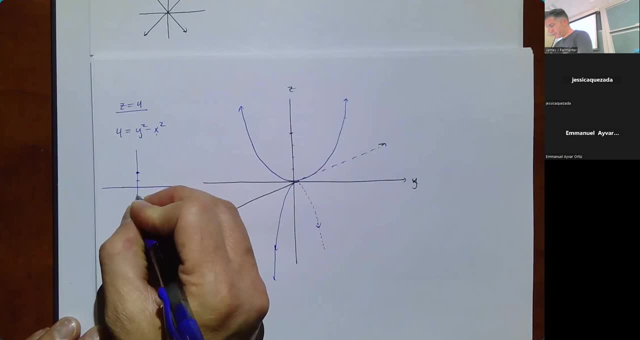 I'm going to get y equal to plus or minus 2 and then if x gets bigger, y can also get bigger. so if x is 1, y is going to be plus or minus root 5. if x is 2, y is plus or minus root 6. 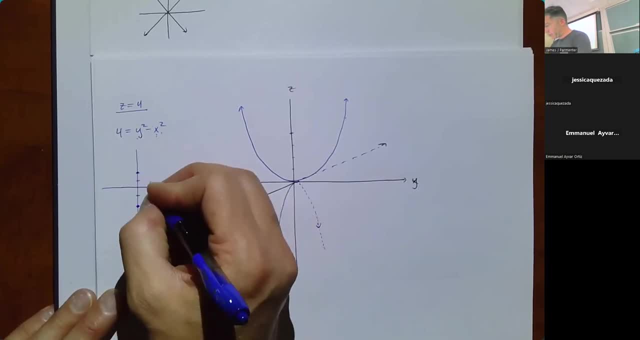 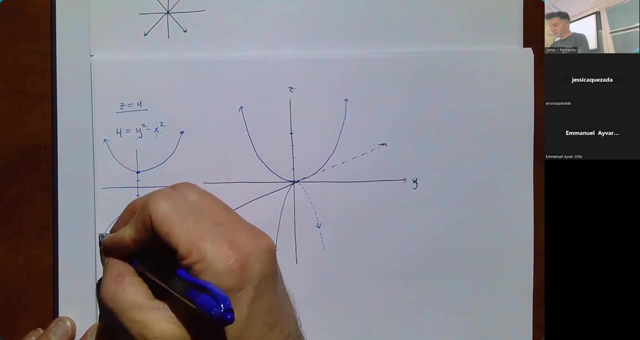 and so on and so on and so on. so what happens here is the x always get larger, the y always also get larger. you get something kind of like that. so I have 9 units of x squared, but I've not done the best job drawing these graphs weirdly have slant asymptotes. 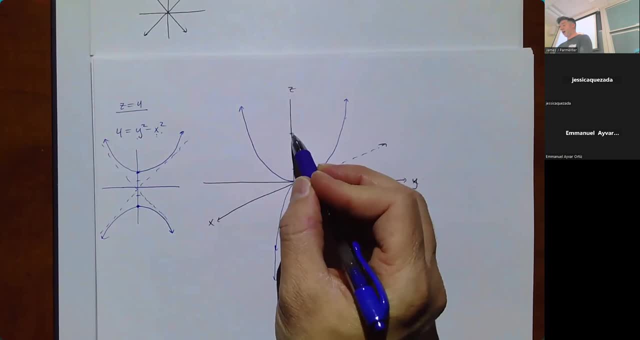 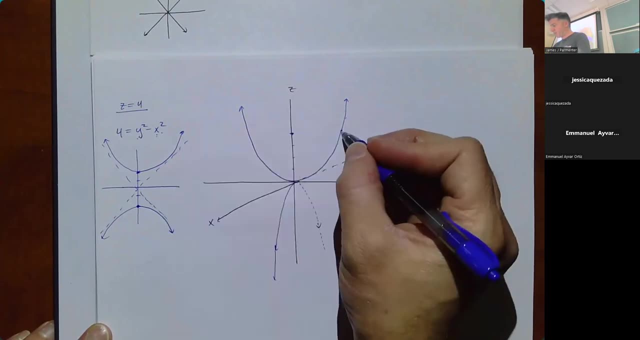 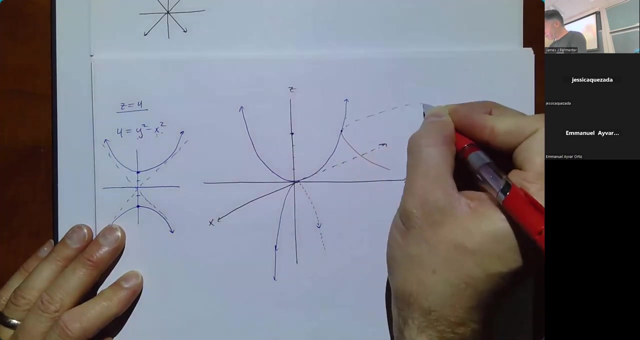 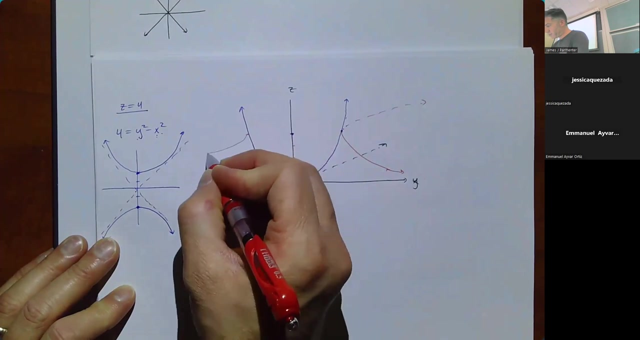 but really the point of this is that if I go up to a height of 2- sorry, a height of 4, check it out from here- I'm going to have this hyperbola. you should use a different color here, going like that and also to the left. 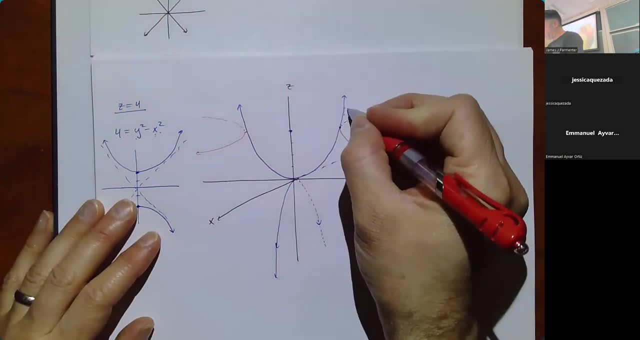 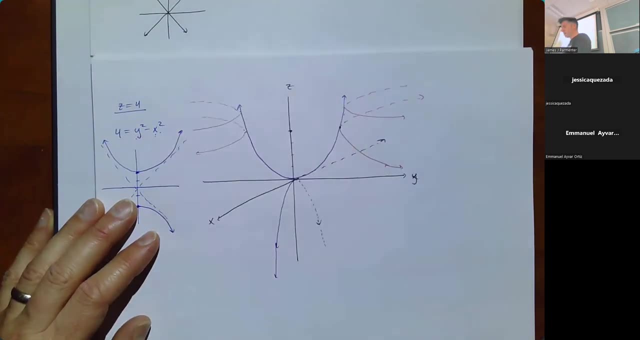 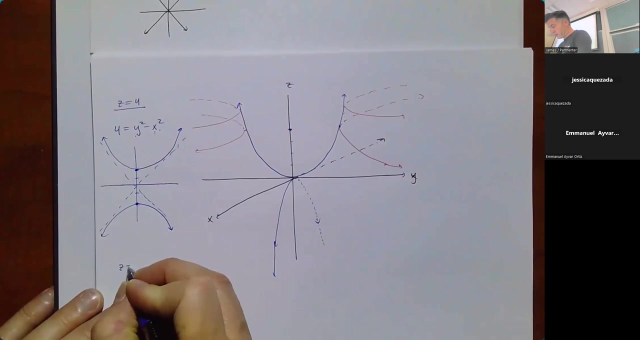 and if I went higher up I'd have another one. so if I keep going up and up and up, I have more hyperbolas. and the same thing also happens if you go down right. if you go down negatively right. if you let z equal say negative 4. 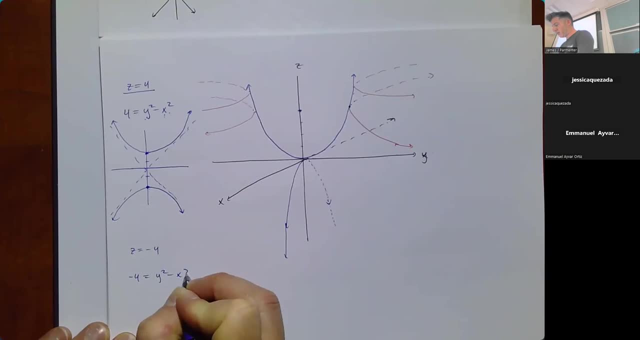 then you have negative 4, equal to y squared minus x squared, which, if we multiply besides by negative 1, we get positive 4 equal to x squared minus y squared. so that's also going to be a hyperbola, but instead of opening up down, 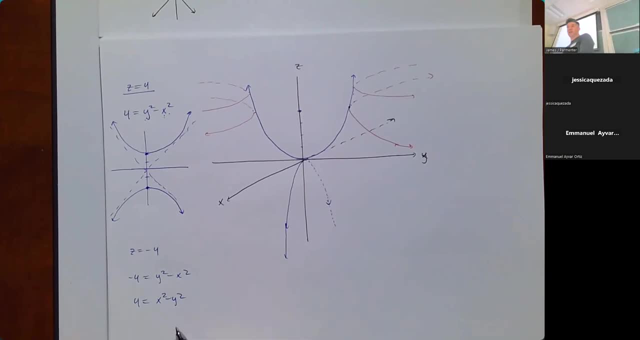 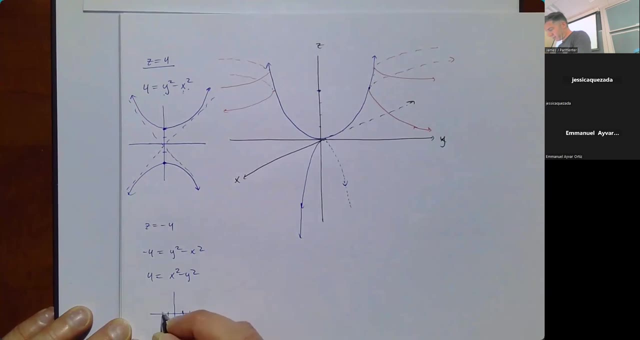 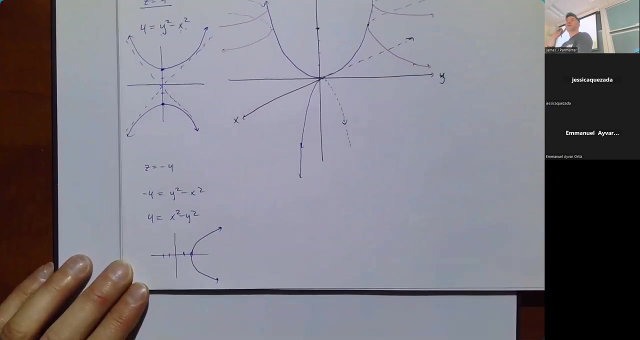 it's going to open left right, because now you get to have the x intercept being plus or minus 2, so this one, this one, looks like this kind of not at all. so yes, thank you. so this is xy. it's still xy again. good call, it's definitely a good idea. 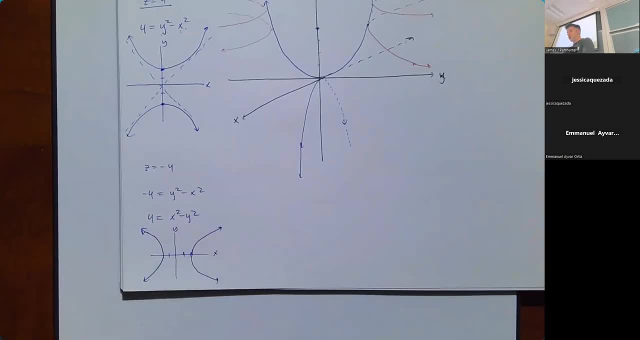 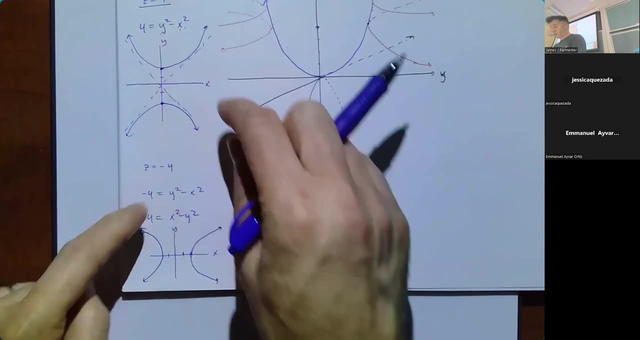 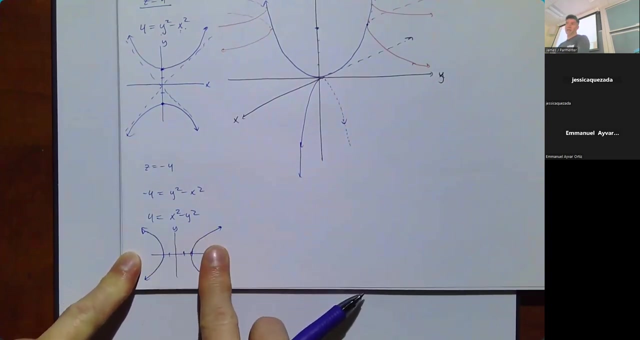 so now, instead of opening to the left and right along the y axis, we're opening to the front and back along the x axis, which I know is not the way this is oriented, but it's the usual way we draw it. so I know it would be nice if we 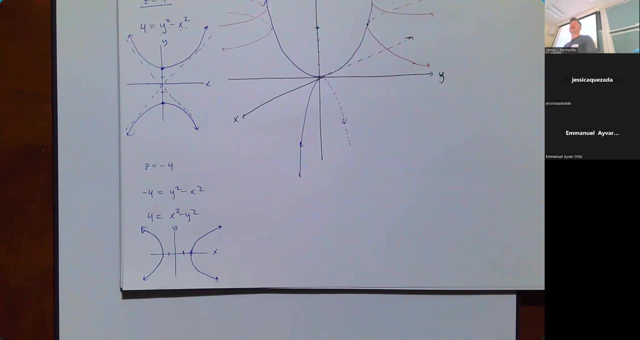 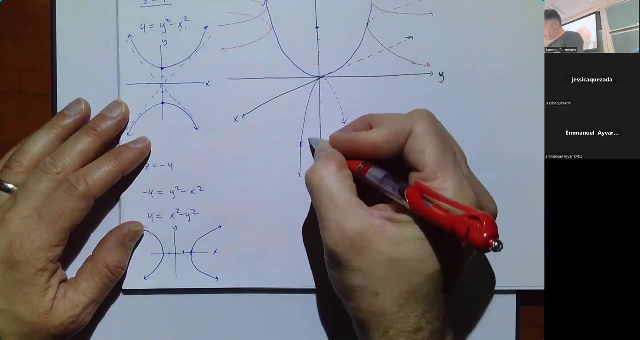 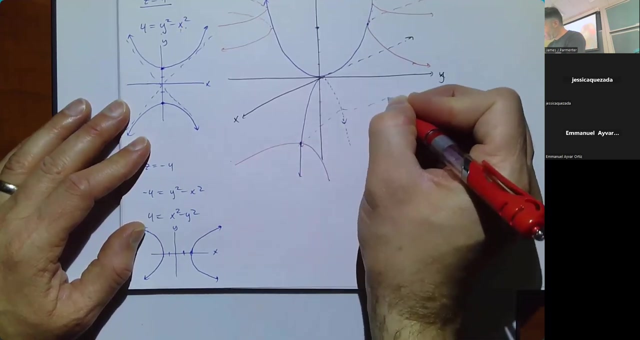 it would be nice if we reoriented this like this, like typically, but it's just not the way it's usually done. so right down here, along here, I'm going to open out towards you and also away from you. so here's what this thing kind of looks like. 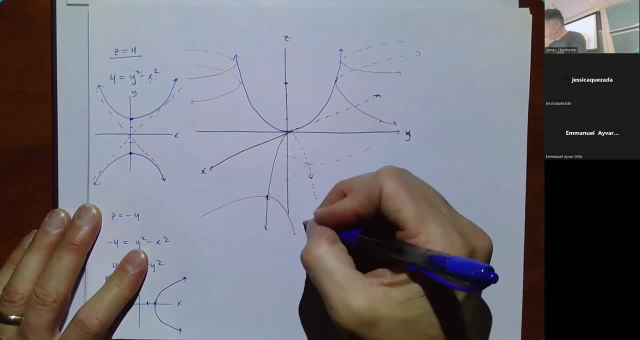 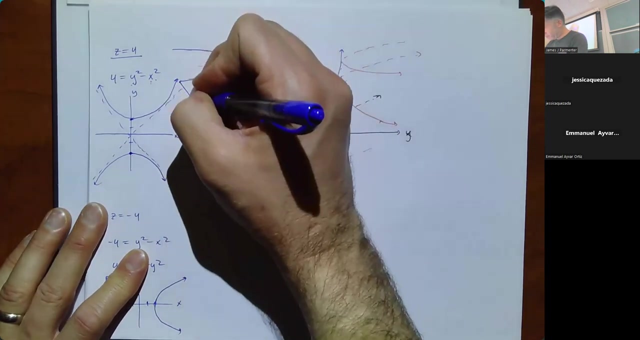 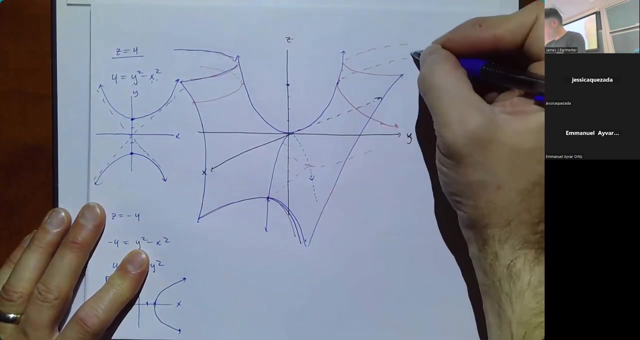 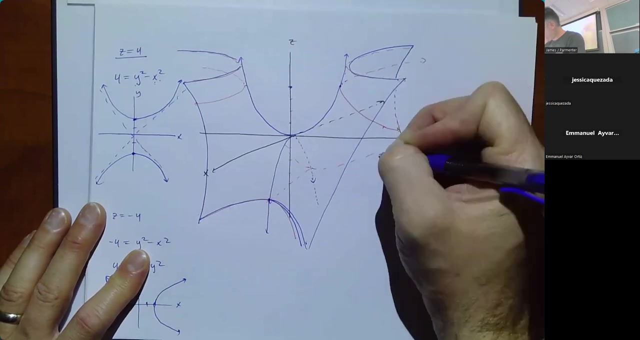 it's actually what's known as a saddle. I've kind of drawn this a little too much of this to make it easy to draw the rest of it. but so you see that you're drawing this and literally called a saddle because it looks like a saddle. 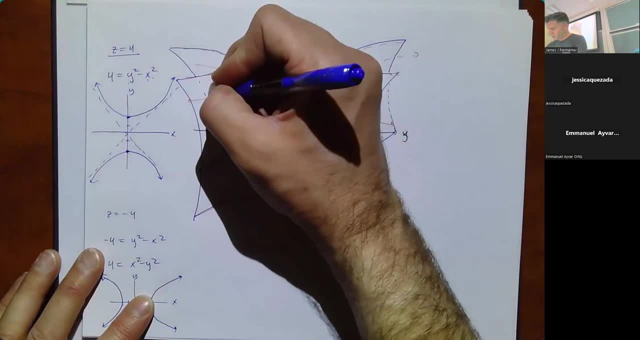 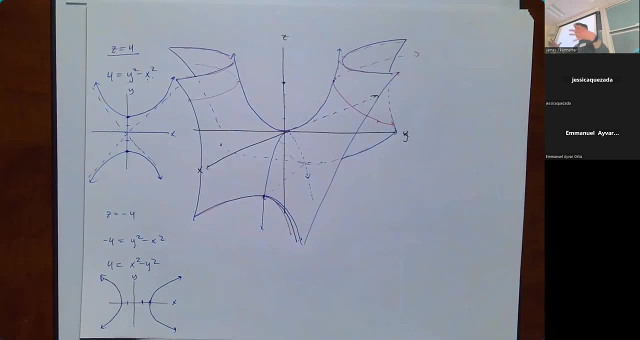 like you could. I mean: yeah, this one's all right and this can be done this way. okay, meet up over here with that, right. it looks like the saddle like you would put on a horse, or if you're out climbing, or I mean hiking, like you know, when you like. 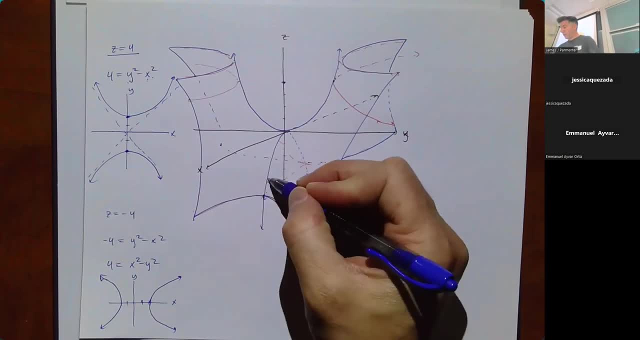 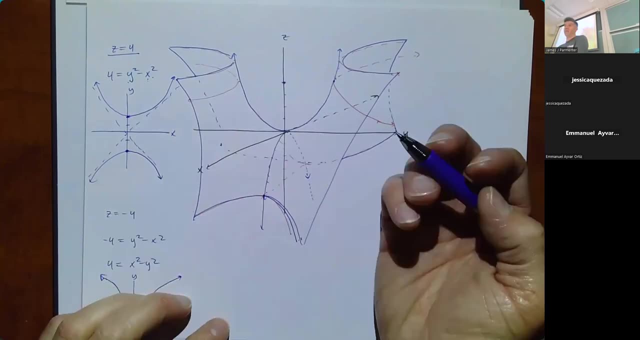 if you ever hike over a hill like you get, you like hiking up, up, up, up, up up and you get to this little point here where you could go over to the other side or you could turn right or left and keep going up and up. that's also called a saddle. 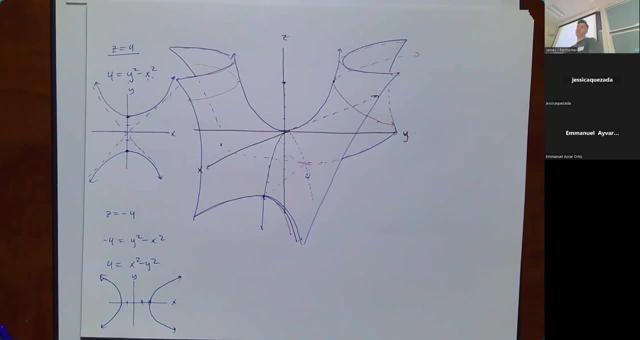 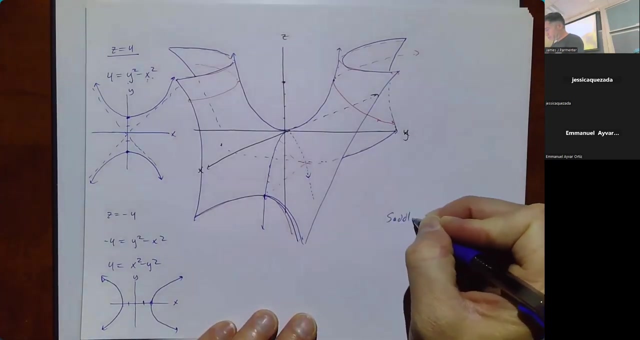 because it's literally a saddle shape. this is a saddle and they're kind of neat, and this is one of the six quadric surfaces that your teacher might expect you to be aware of. so generally, there's a few others. yeah, we got that, so let's talk about a couple other ones. 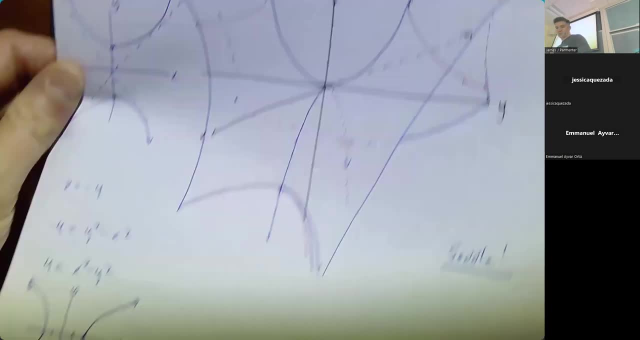 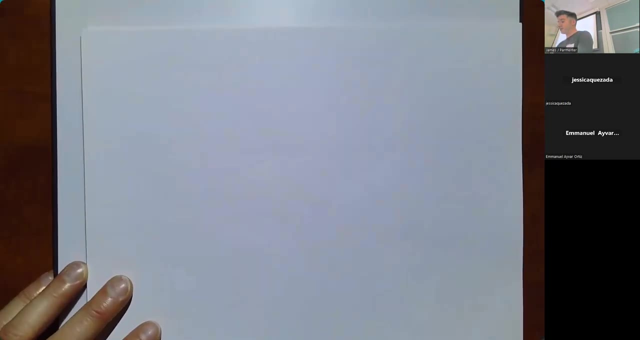 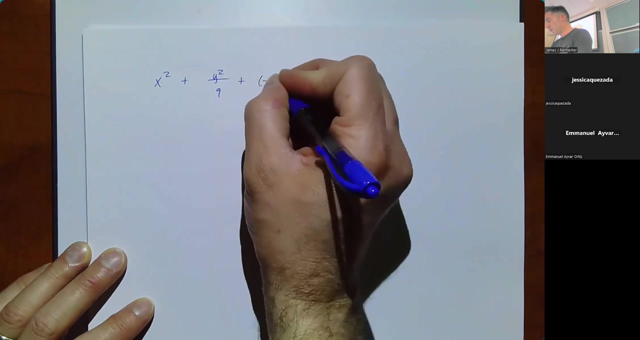 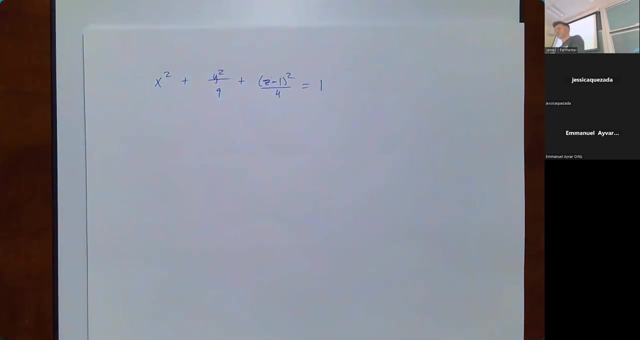 just because they're neat. so here's another quadric surface, maybe the one that's a little bit easier to visualize: x squared plus y squared over nine, plus z minus one squared over four, equal to one. this one almost has the hallmarks of a sphere, except. 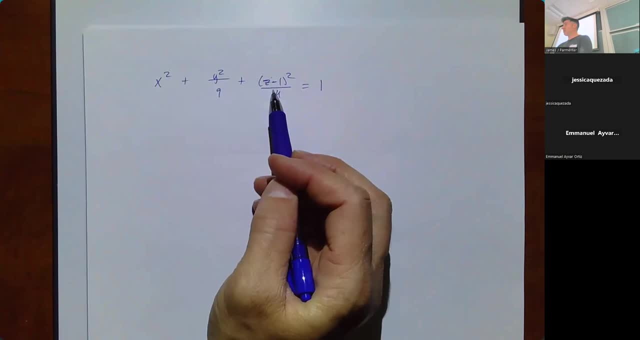 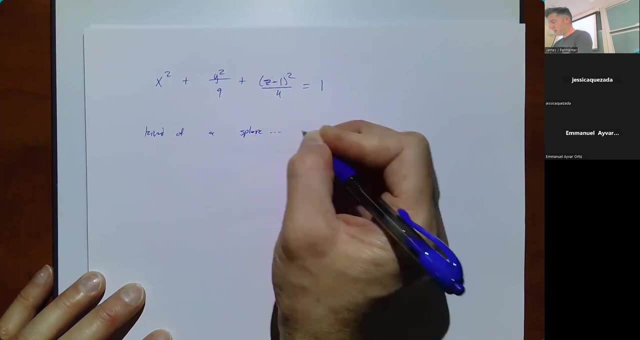 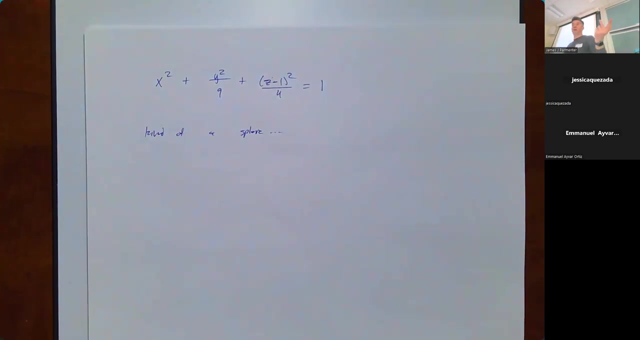 we don't have the same coefficients on x squared, y squared and c squared. this is kind of a sphere, but it's actually called a. what is it? an ellipsoid, an ellipsoid, so it's like an ellipse, except it's kind of been rotated around the other axis. 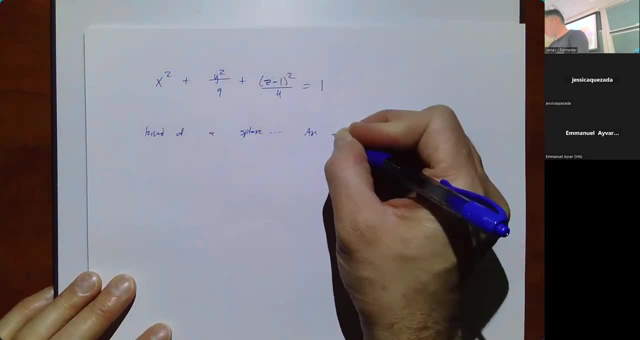 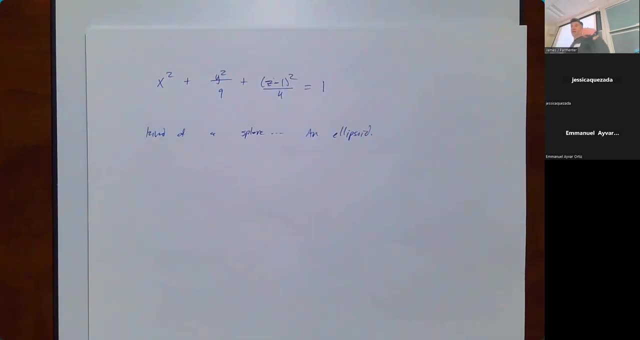 this is called an ellipsoid or, as I would rather say, a sphere, is an ellipsoid where all of your axes happen to have the same length. this ellipsoid- well, let's talk about the center. center of this ellipsoid- is going to be x equal to zero. 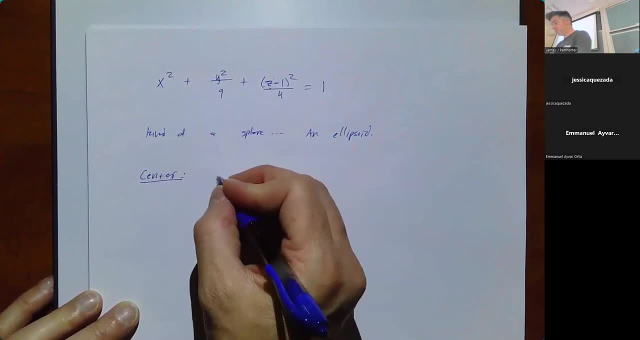 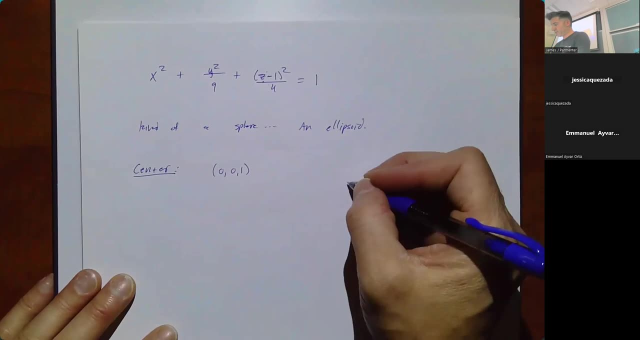 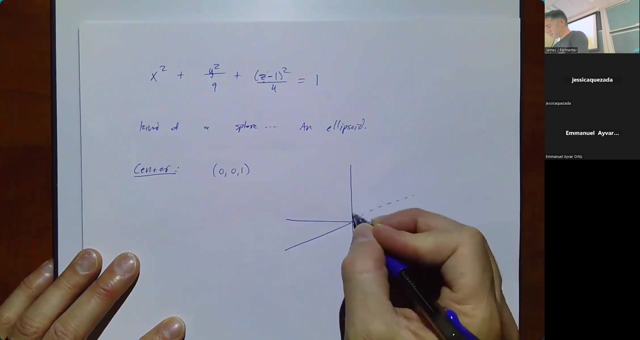 y equal to zero and z equal to one, which is maybe less than i do for drawing. there's the center of my ellipsoid, and then we can kind of find all of this, and then we can kind of find all of the endpoints of the different major and minor axes. 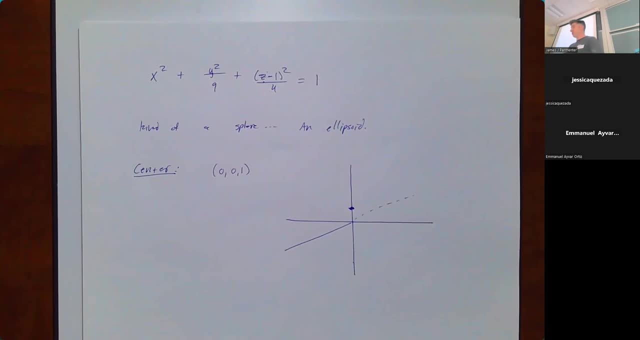 by kind of seeing what x, y and z would need to equal when the other ones would be zero. so if, yeah, sure, if x and y were both zero, z could be as big as three and as small as negative one. so here's what I'm doing. 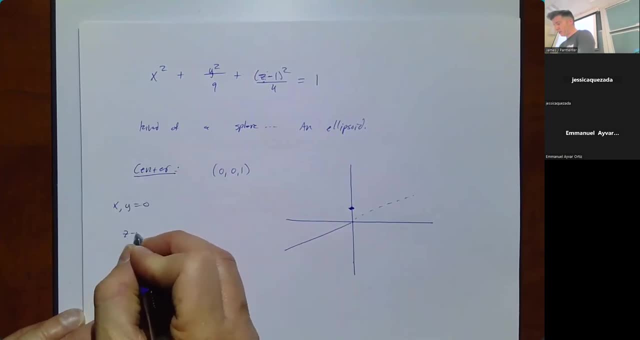 if I set x and y equal to zero and I have z minus one squared over four equal to one, I have z minus one squared equal to four. I have z minus one equal to plus or minus two. so z is equal to one, plus or minus two. 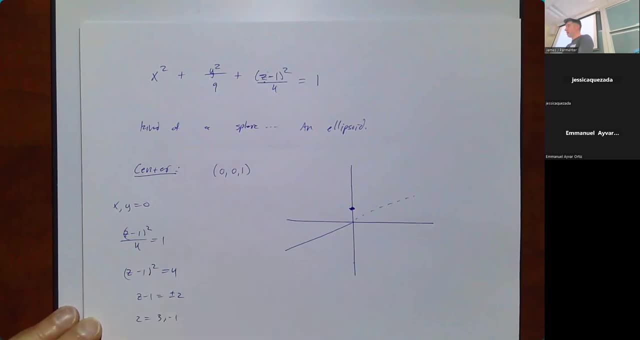 so that's three or negative one. so basically, from the center I can go up to or down to, and I'm going to do the same thing for the other variables, except I should be a little more careful. I'm not setting everything to zero exactly because I picked a different center. 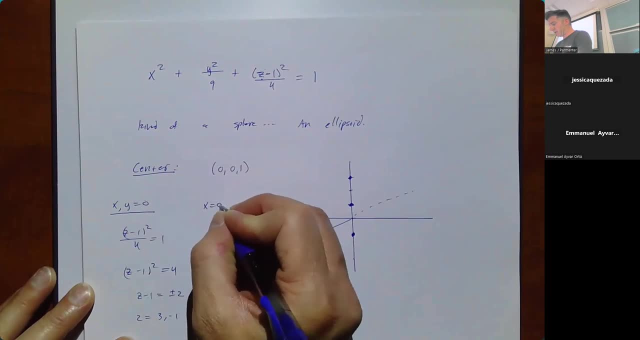 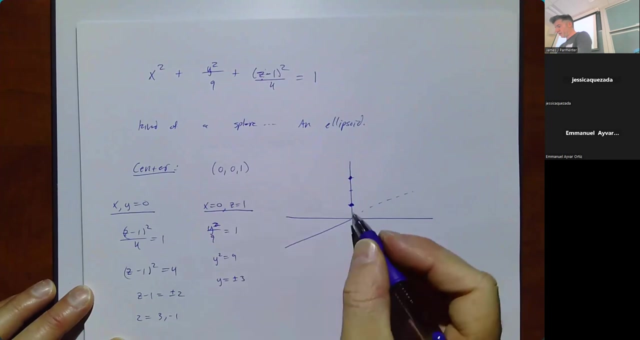 so I really should say I'm going to set x equal to zero and z equal to one. if I do that, I'm left with y squared over nine equal to one, which means y squared is equal to nine. y is plus or minus three. so from the center I can go. 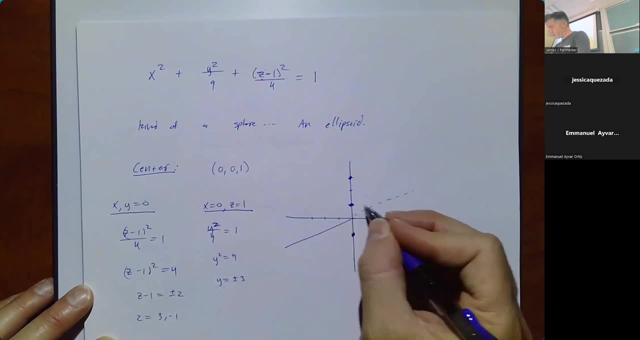 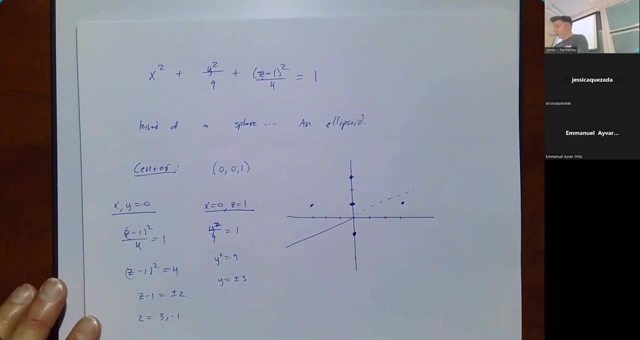 three to the right and three to the left, and actually I'm going to do myself a favor here. I'm just going to draw this oval right now. so here's my oval in the yz plane. let me see how well I can draw an oval here. 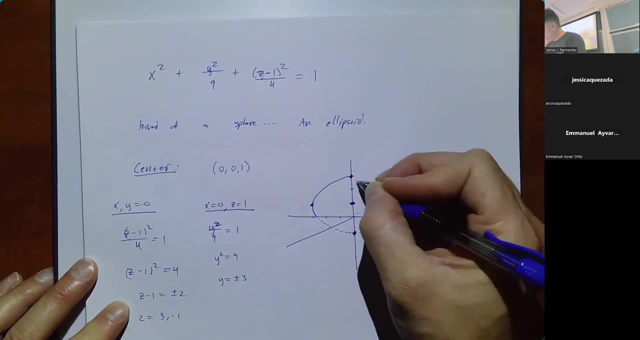 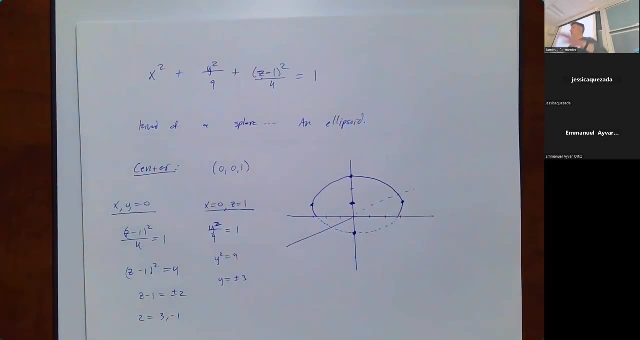 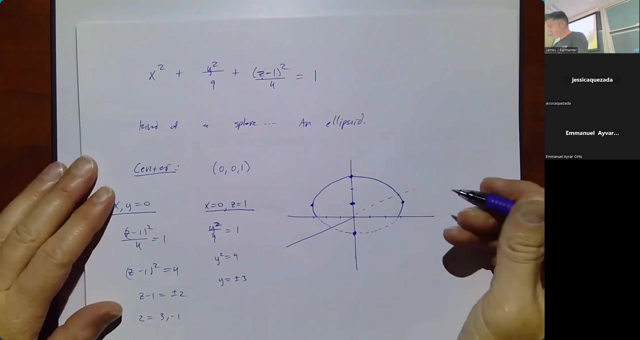 pretty good, not the worst thing I've ever drawn. and then finally, not in the yz, not in the xy plane, but in the shifted up one from the xy plane. sorry, I'm going a little ahead of myself here. so setting z equal to one and y equal to zero. 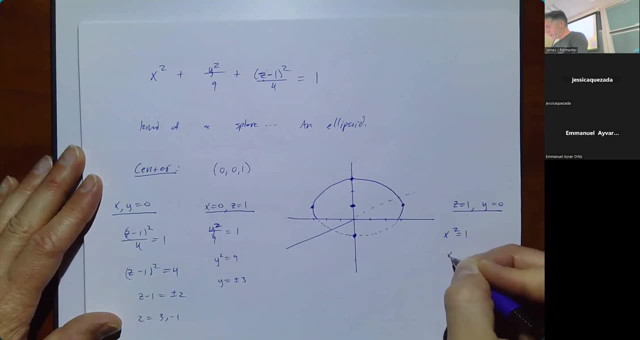 I'm going to get x squared equal to one. x is plus or minus one, so this is one that's going to be kind of hard to draw. I'm going to come out one in this direction, right there. I'm going to go one back. so just to clarify what I'm doing there. 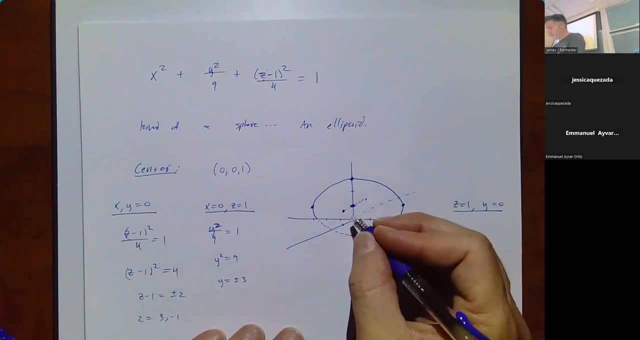 because I know it looks not lovely. I'm saying, from this point here, from the point where y equals zero and z equals one, I'm moving forward one in the x direction and backwards one in the negative x direction and I'm going to try and draw the oval. that kind of hits that. 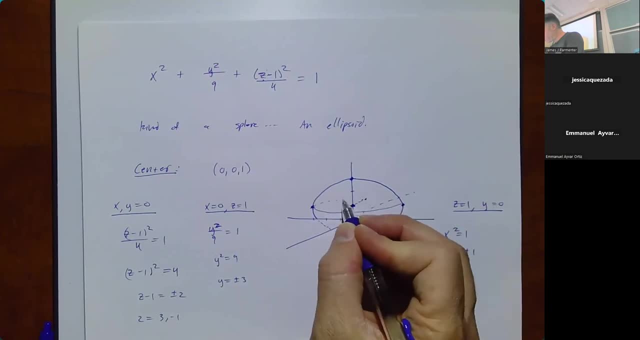 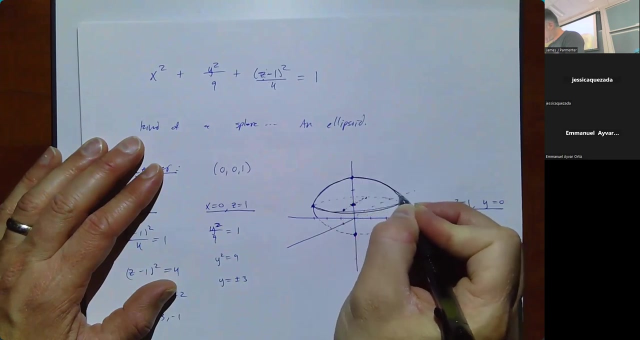 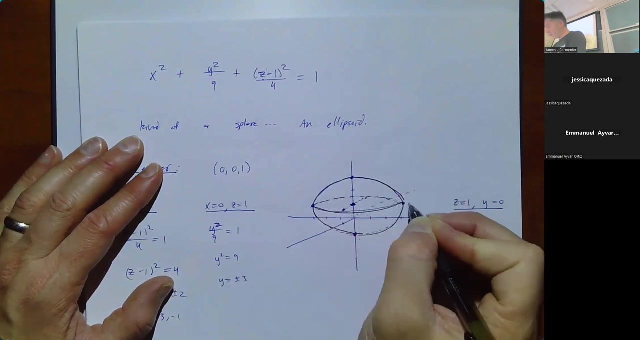 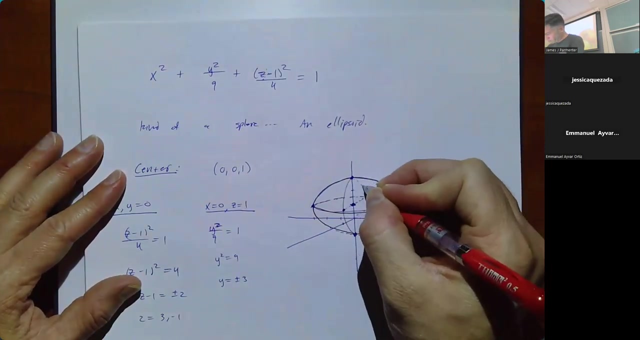 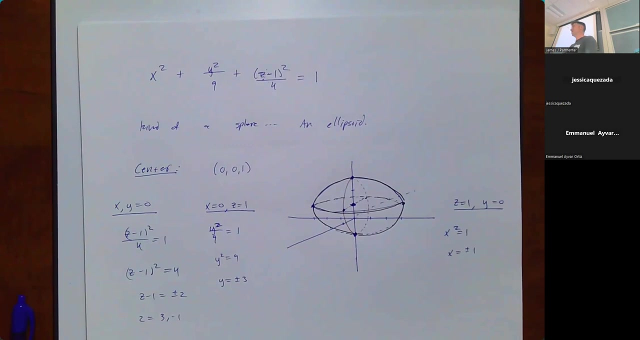 mark as well, and I'm going to try and draw the oval that kind of hits that mark as well. so here's our ellipsoid, and the one I haven't drawn yet, which I'm about to, is this one right here. so those are well, two of those are traces. 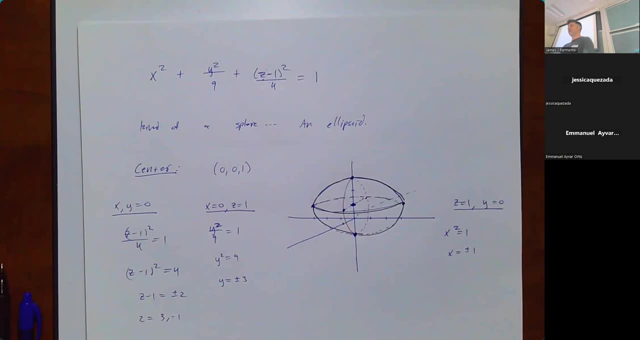 one of those is a level curve. so what's the difference between a trace and a level curve? not a lot, actually, except the trace specifically refers to being in one of the three coordinate planes, either the xy, the xz or the yz, whereas a level curve 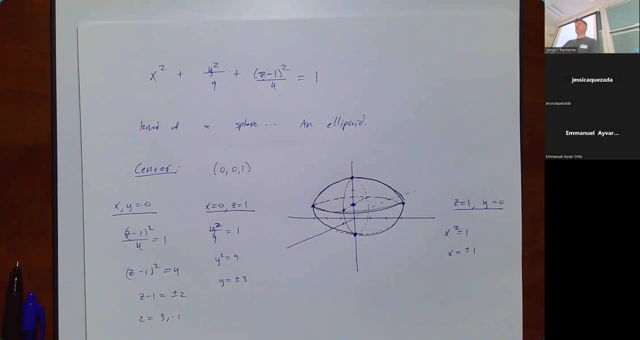 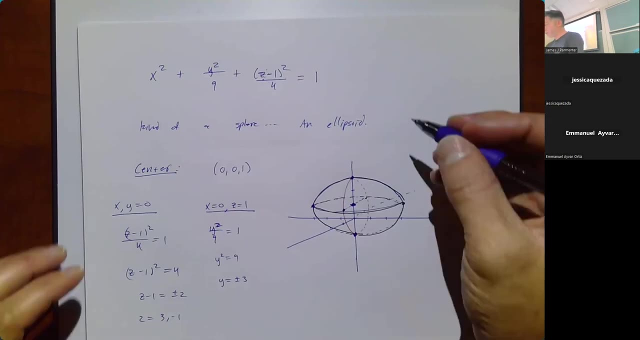 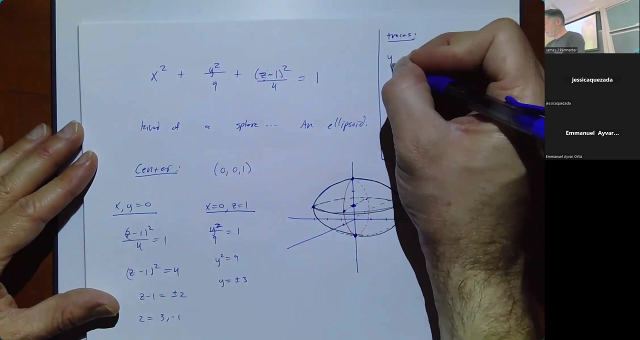 usually means you're setting z equal to a specific value and seeing what things look like at that particular height. so just to kind of say a little bit more here, our trace is. our trace is in the yz plane. we're setting x equal to zero, we're getting y squared. 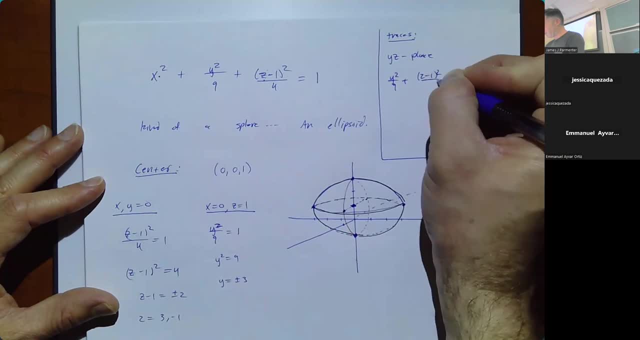 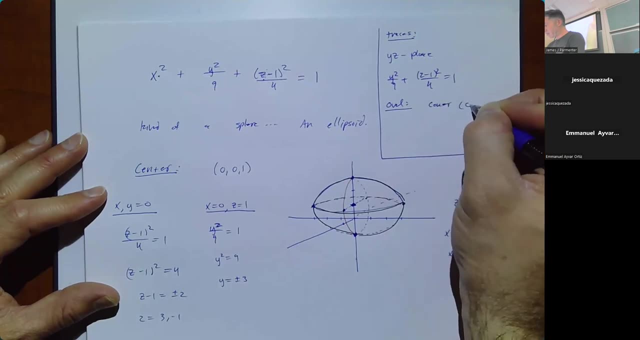 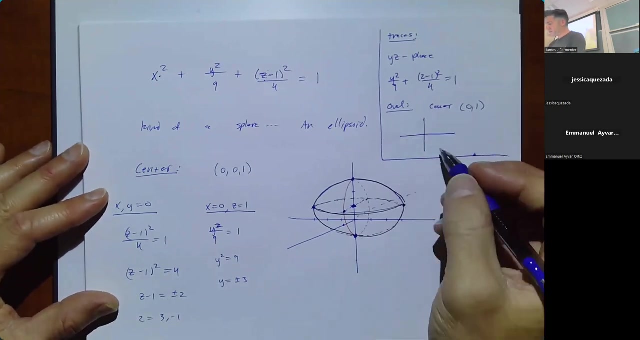 over nine plus z minus one, squared over four, equal to one, and that's an oval. the center is zero comma one, and it's well, in fact, let's draw it. I've already kind of drawn it, though. so there's zero one and you get to go. 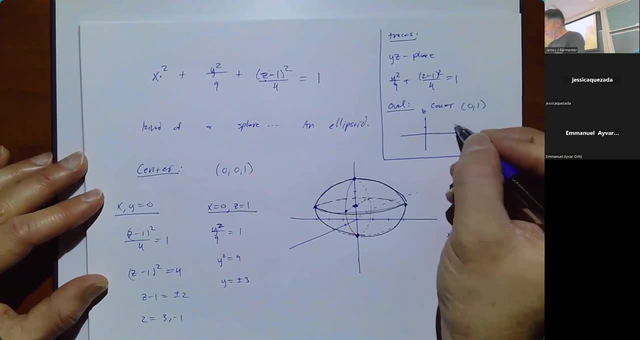 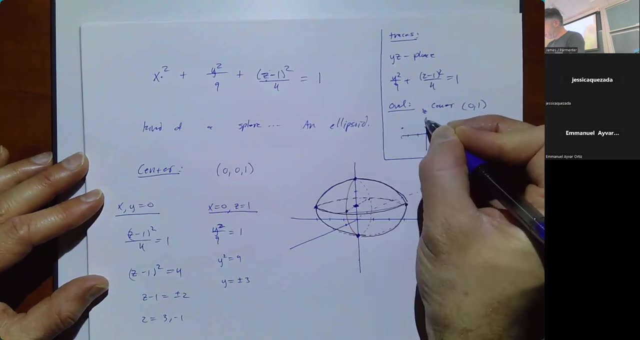 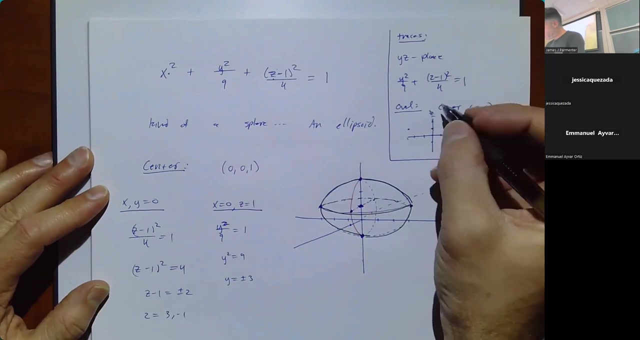 sorry that's. I feel like it's really small here. I guess it's not the smallest thing. you're going three in the y direction and two in the z direction. let's try and use the same color, james, so that, right there, that's this trace, right here. 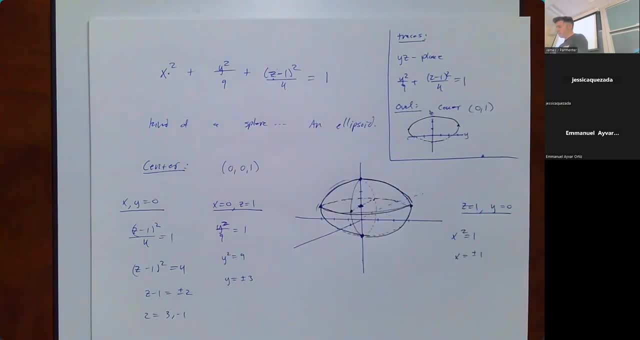 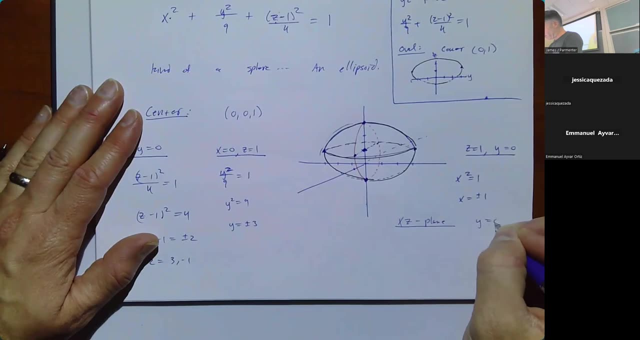 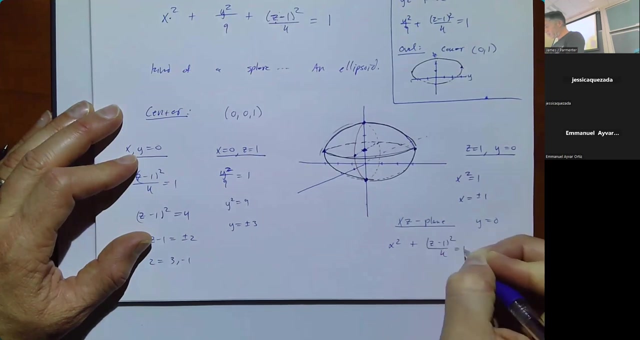 and then similarly in the xz plane. if we set y equal to zero, we're just getting the trace where x squared plus z minus one squared over four, is equal to one, which ends up being this red oval here. right, you're still at the same center. 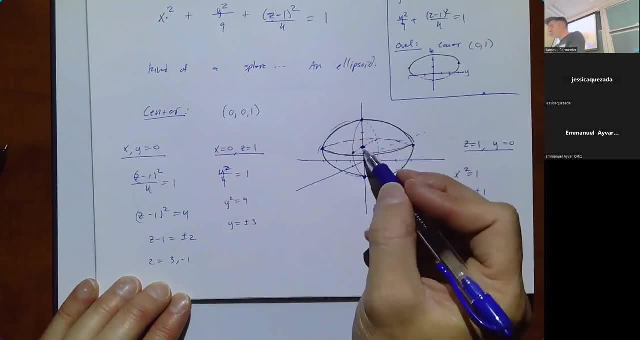 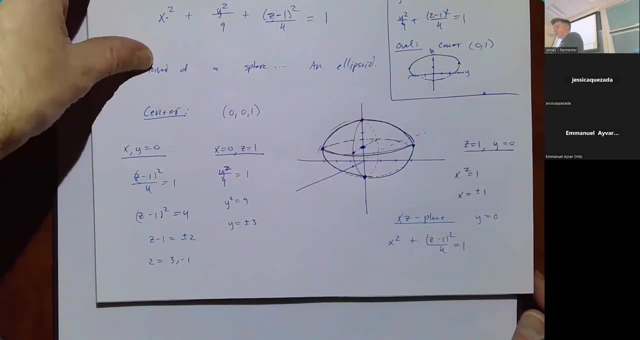 and then you're going two in the z direction, two up and two down, and one in the x direction and then in the xy plane. things are kind of weird. you could find the trace in the xy plane. if we do that, you're going to get a slightly 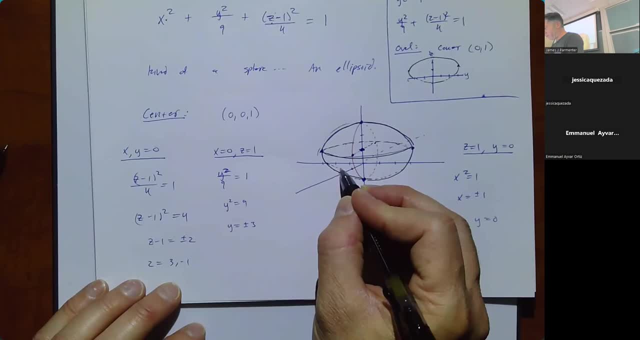 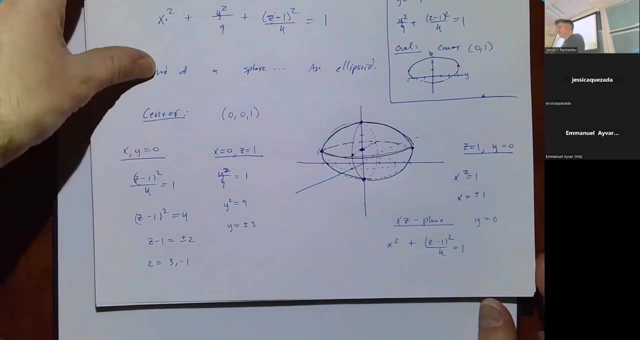 you're actually going to get something we haven't drawn, which is like this smaller oval here, because that's what's happening in the xy plane and we could find that if we needed to. but really what's kind of more useful for drawing this picture is what's happening when z equals one. 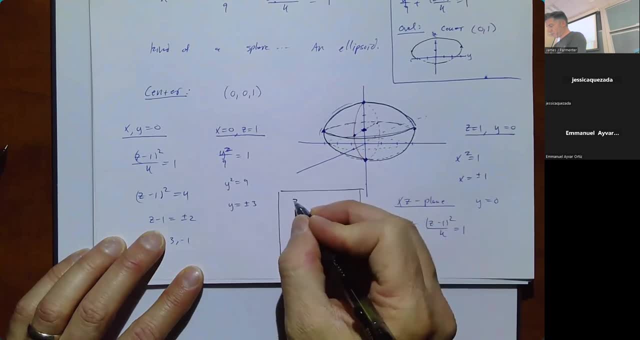 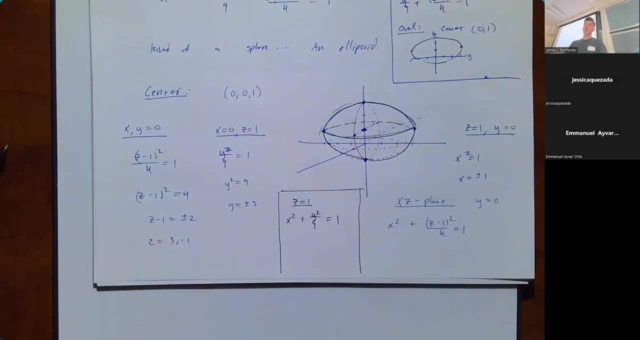 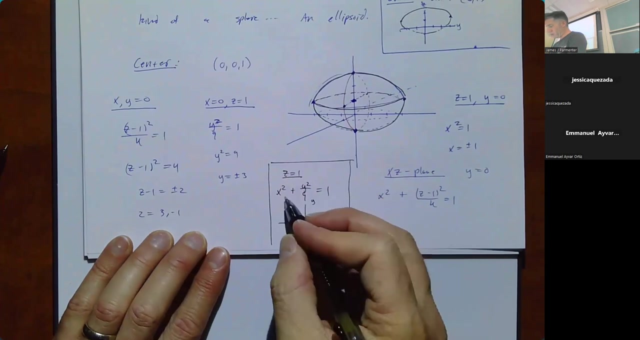 and then so z equals one. then we're left with x squared plus y squared over. nine equals one. that's another oval where the center is the origin, and you can go one in the x. I've given myself not nearly enough room here. we can go one in the x direction. 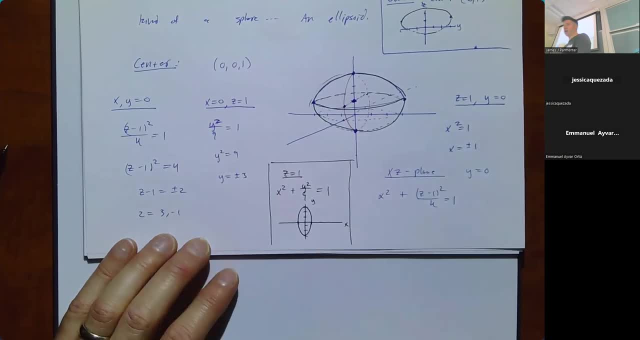 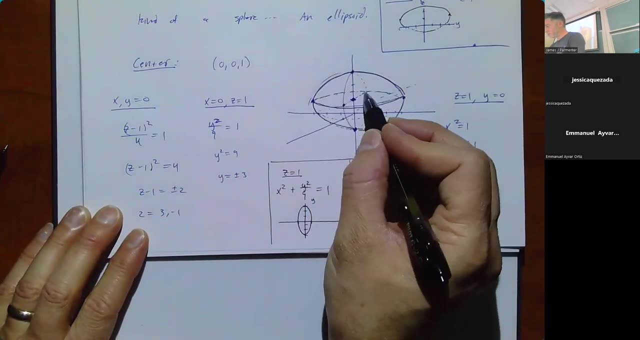 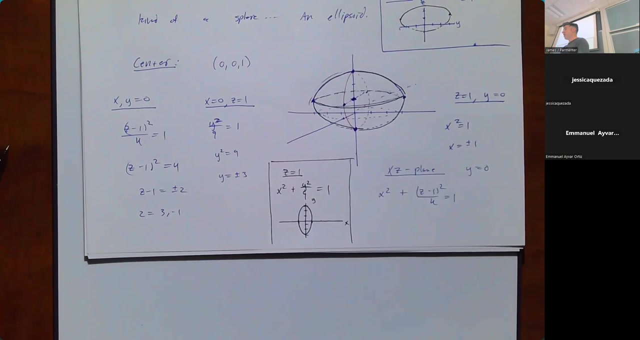 and three in the y direction, which is that red one there? no, no, sorry, not the red one, this flat one here, apologies. so graphing in 3D is hard, but it doesn't have to be super duper hard. um yeah, what the other thing I would say? 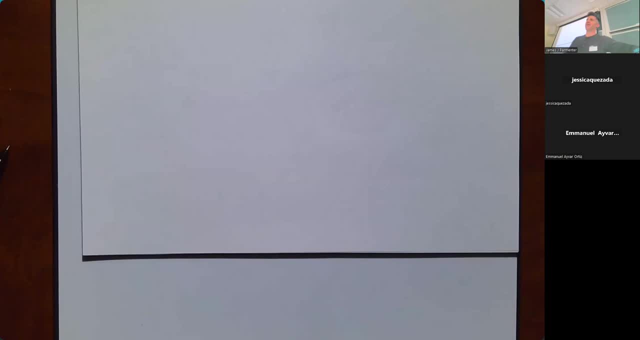 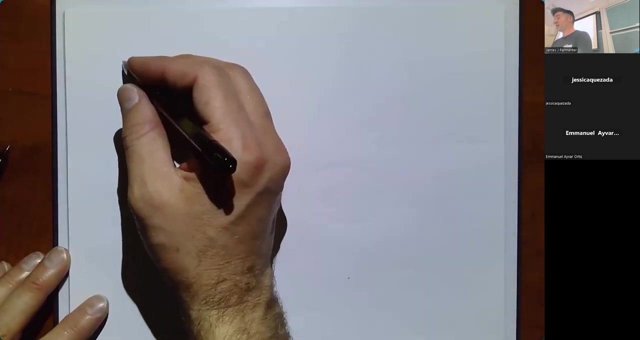 is that? what would I say? kind of think about what I would like. I would say that your, if you're trying to graph things in 3D, I think starting with finding I know what I should say in this last minute here. something I kind of skipped over which is important is: 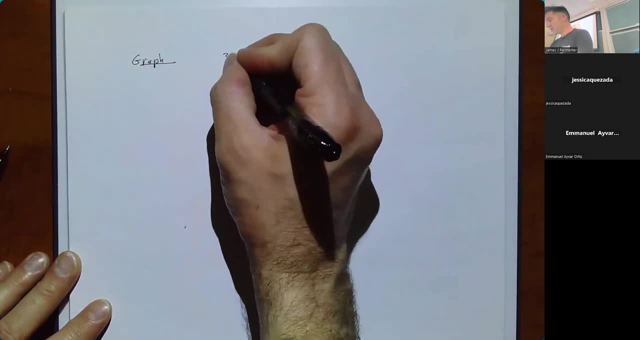 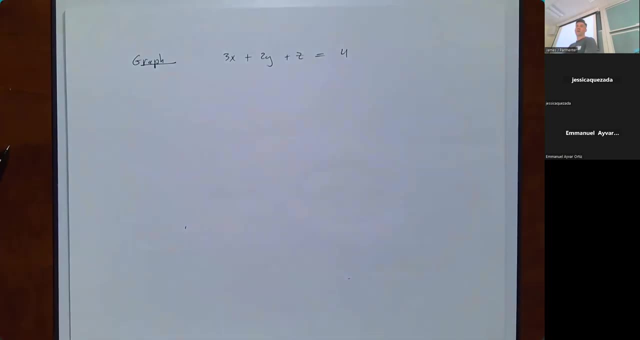 let's say we wanted to graph the following equation and I got a minute: 3x plus 2y plus z, equal to four. in this equation, since everything is linear right, every variable is raised to a first power. that's almost always a sure sign that we have a plane. 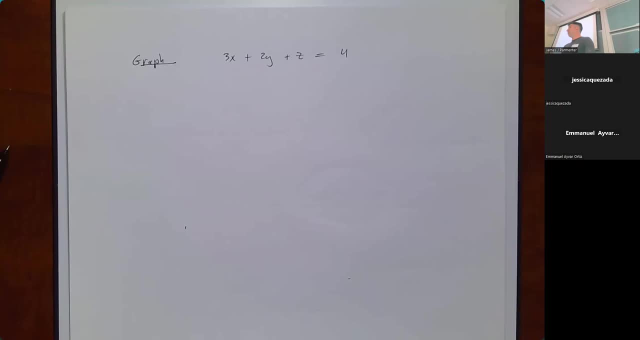 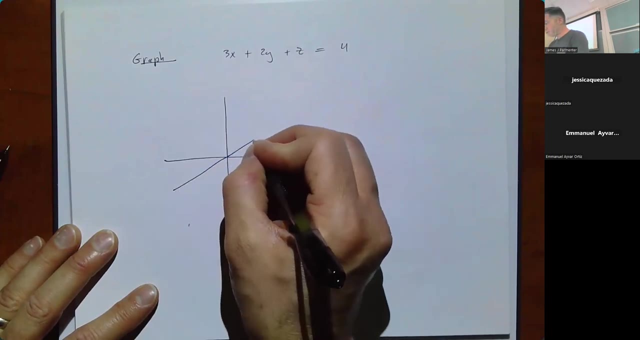 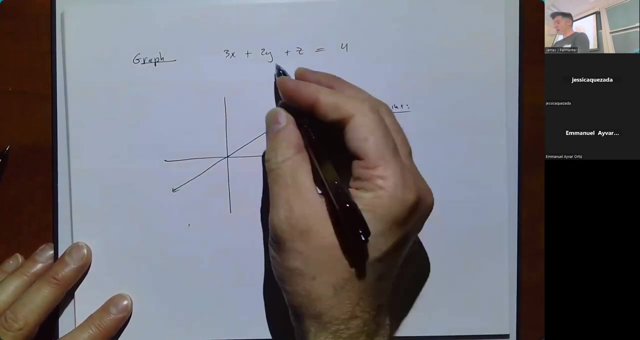 when you draw a plane you really just have to draw or find three points and connect them up. so if I was drawing this plane, I wouldn't worry about my traces. I would find my x, y and z intercepts. so the x intercept, I'm going to set y and z equal to zero. 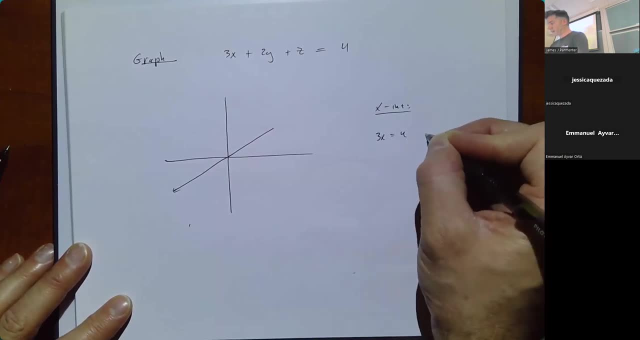 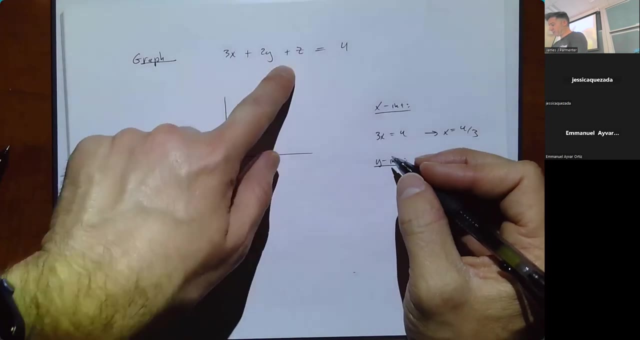 I'm going to get three x equal to four of x equal to four thirds. y intercept: same deal. set x and z equal to zero. we're going to get two y's equal to zero. set y equal to four. we're going to get y equal to two. 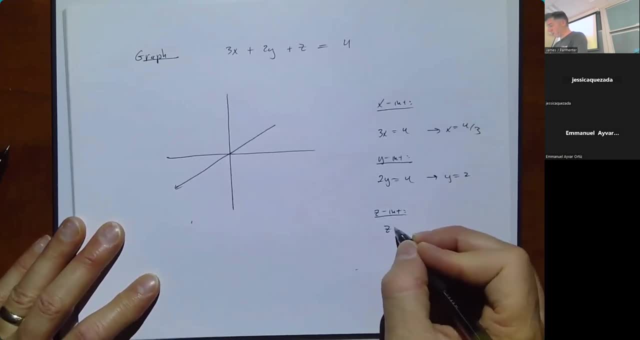 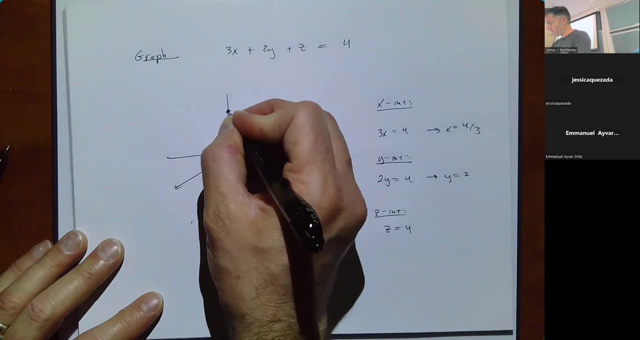 and for my z intercept, we're going to set x and y equal to zero. we're going to get z equal to four, and then you plot those four, those three points. there's z equal to four, there's y equal to two, x equal to four thirds.